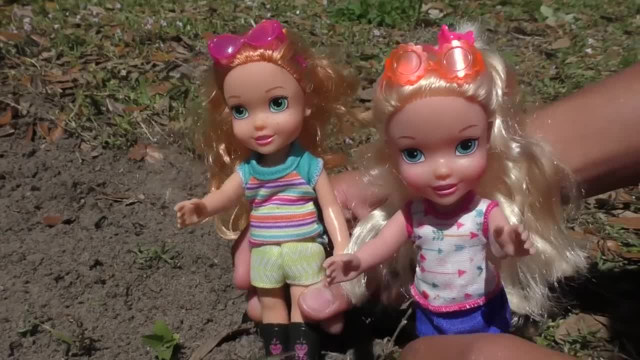 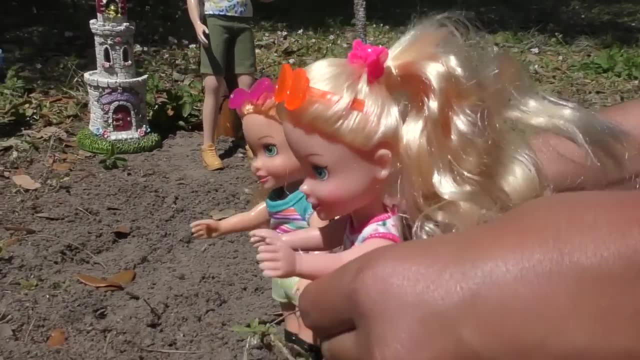 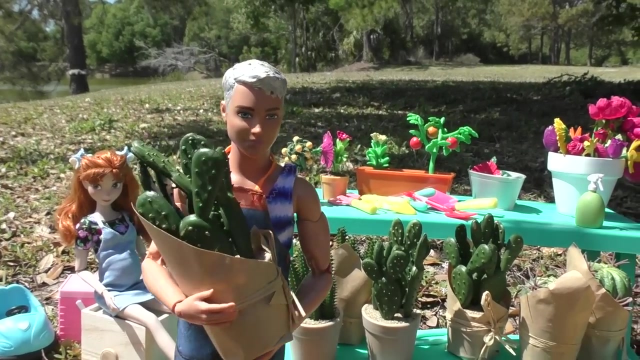 We love our spring outfits and we have our boots, because it's time to plant. Yes, mommy, mommy, I like them girls. Oh, Jack, are you done bringing all the plants? This is the last cactus and now we can start planting. 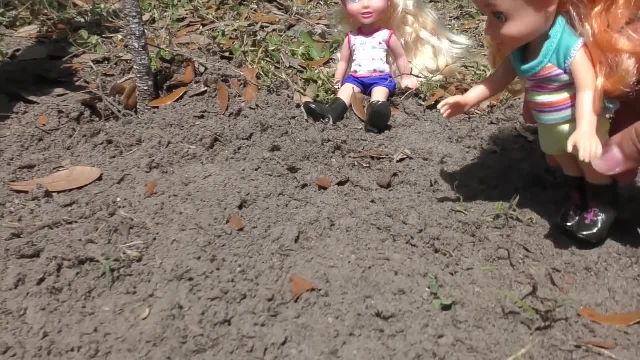 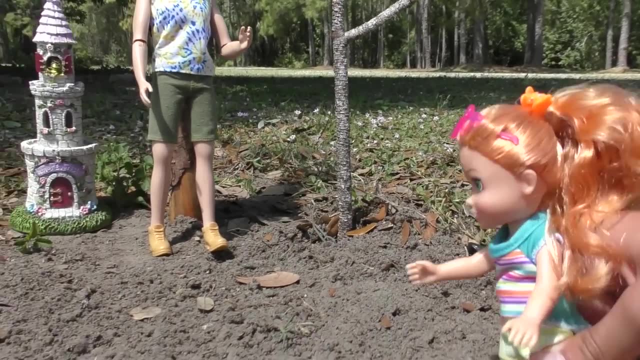 Did you hear that, girls? Yep, Whoa, there are ants over here in the dirt, ready to plant. Wait, where's Biscuit, Biscuit, where are you Biscuit? I see it. Come here, Biscuit. it's time to plant. 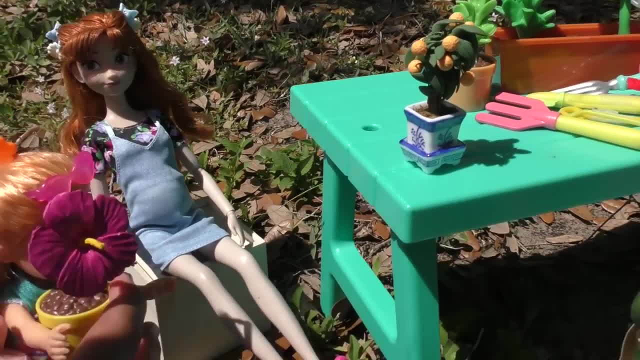 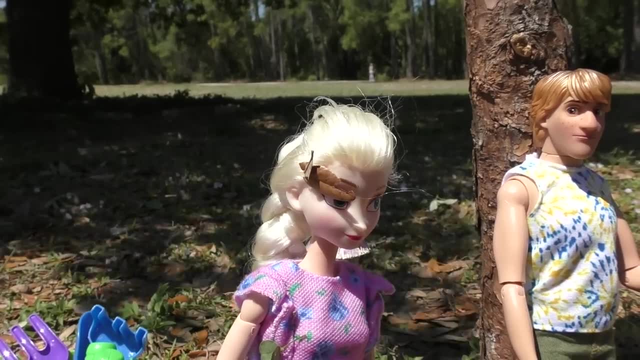 And Tangie. Yep, Tangie, come with me too. Elsa, you have leaves on you. A natural earring? Oh yeah, it does look like it. Can you help me plant a biscuit? Well, hold on, we have a plan. 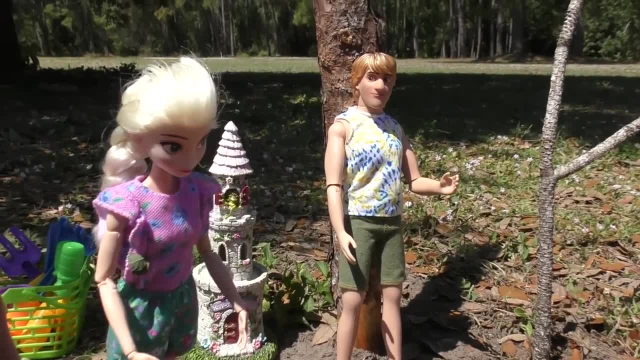 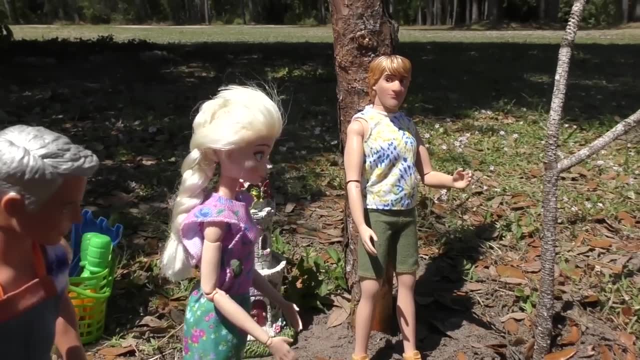 What plan? Well, first we're going to put a fence around this patch of dirt right here. see, This is where we're going to plant all the plants. Oh yeah, perfect. And then we'll put the cactuses and then the small flowers. 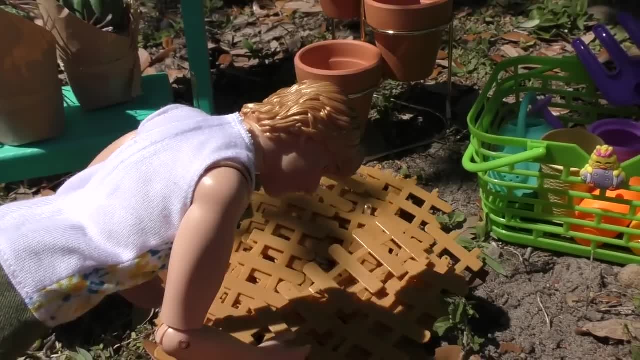 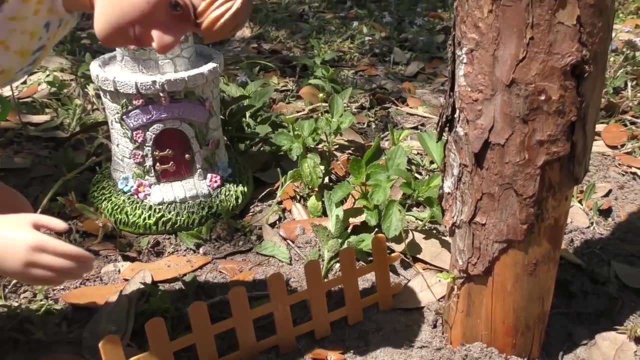 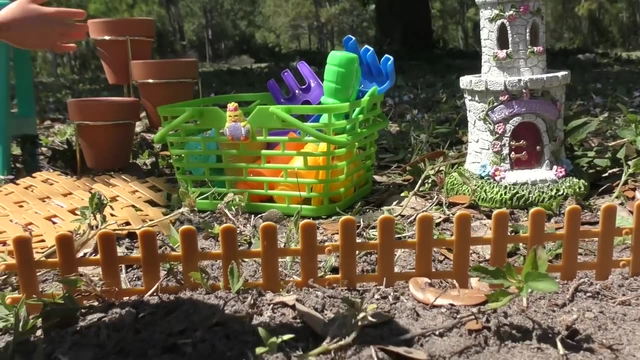 So Biscuit can wait. Yep, Okay, I'm going to start from here And I'll help you. Kristoff, Thank you. Here come the next pieces And snap it's all together. The next side will be coming like this: 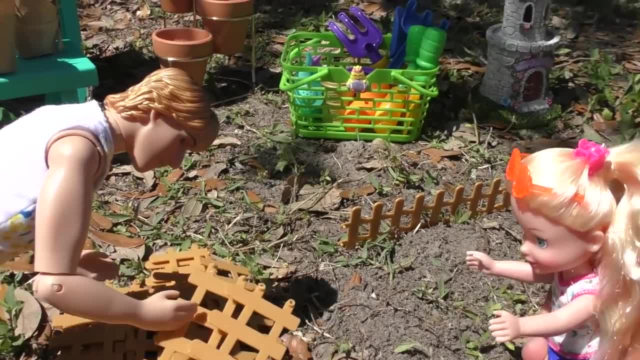 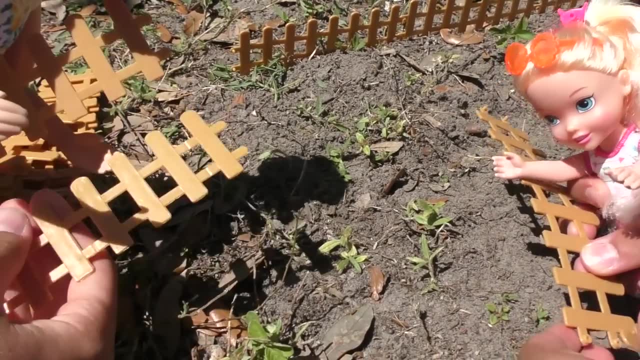 Uncle Kristoff, can I snap some fence pieces? I think you could try. Yes, It's so satisfying. Okay, here's the holes And snap, just like that. Mm-hmm, Good job. Okay, I did it. 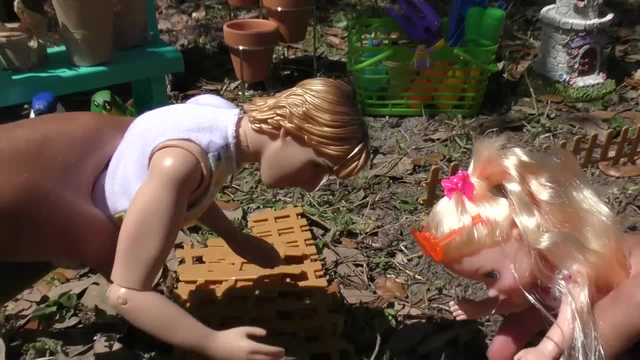 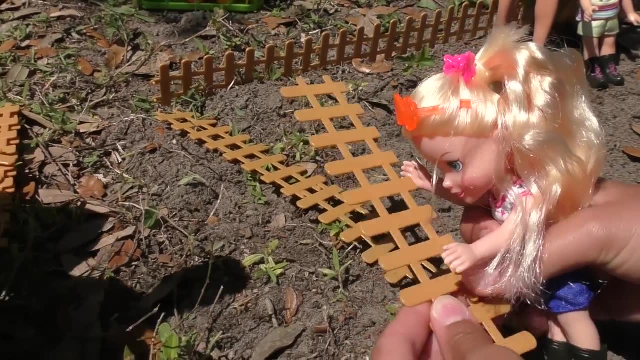 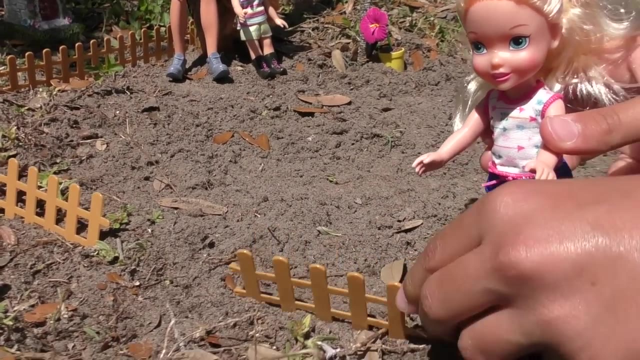 Yes, Mm-hmm. Next, Can you snap this way And click. Thank you, Mm-hmm. I'm going to leave a space so we can enter Mm-hmm And it can become our little house. 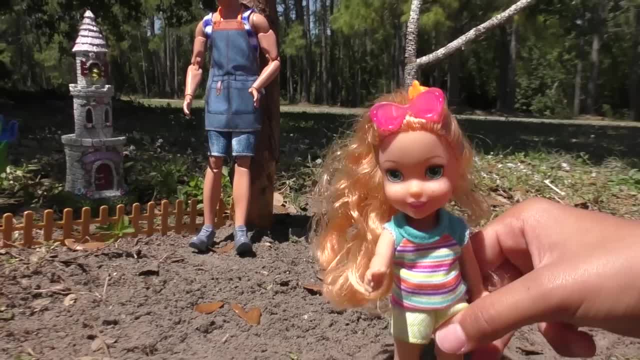 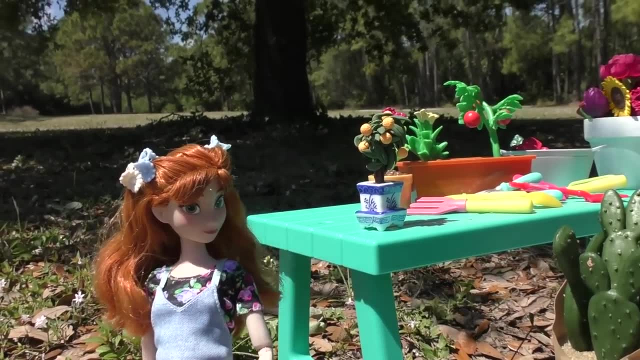 Mommy, can we please make this our house now? It's a great idea. Well, it is like a house, but it's only for the plants and there's no roof. Well, for us it is like a mini house, but it can also be a plant house. 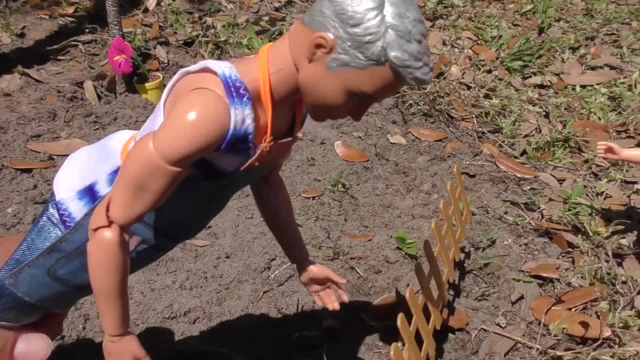 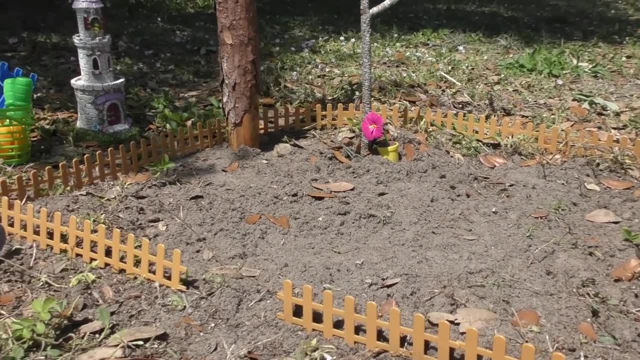 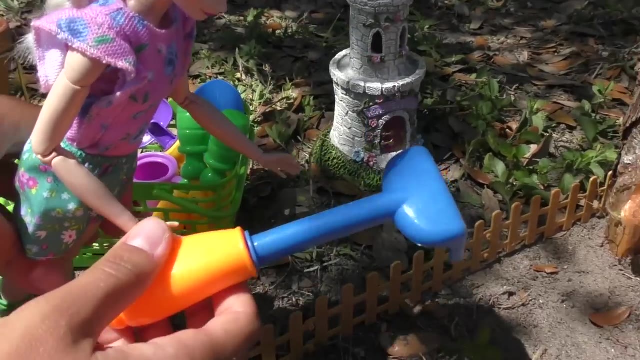 Yeah, I like it. Excuse me, girls, I'm going to put this piece of fence over here. Okay, I like this patch of land we made. Now it's all surrounded so we can get planting. Yep, Now we're going to get the rake to make the soil smooth. 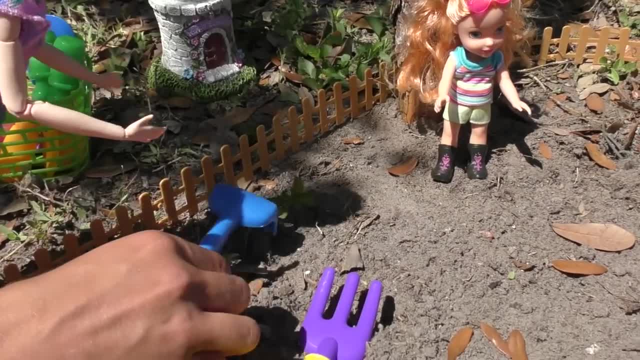 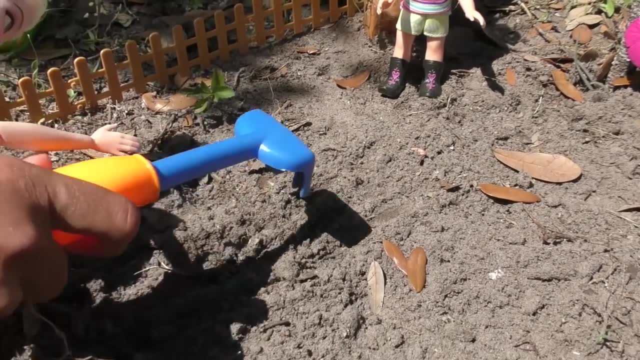 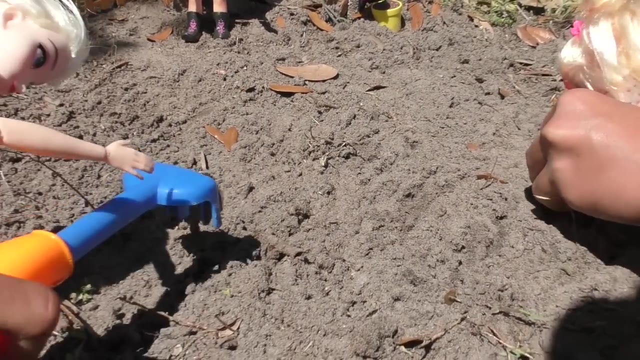 And girls, you can use this one if you want. Yes, Mm-hmm, So do I just grab, like this, So you go only from one direction, from up down, like this. Okay, Gardening is so relaxing. 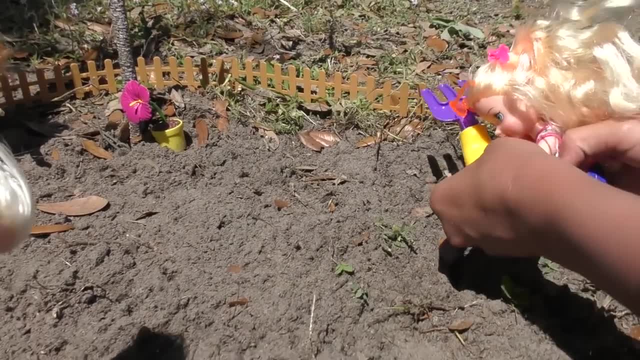 Yeah, It's satisfying too, And at the end it will be filled with beautiful plants. I'm starting to bring the cactuses. Is this a good spot? Yep, This is perfect. I'll plant them over here. So now we need a shovel. 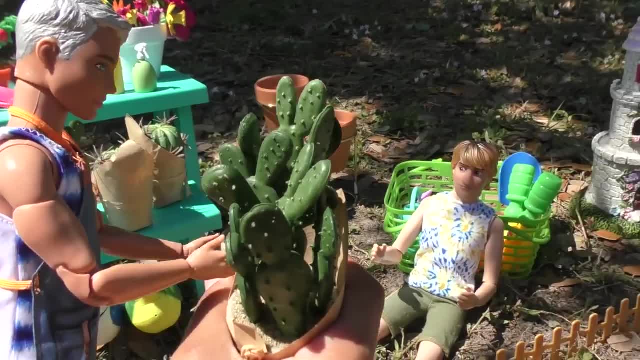 I'll get it for you. Here you go. Okay, girls, Watch and learn. This is how you're going to plant. First, you dig a hole, Dig, dig, dig- Oh, Big enough for the plant to enter. 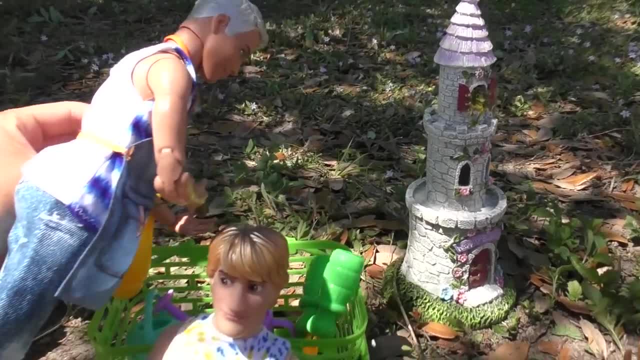 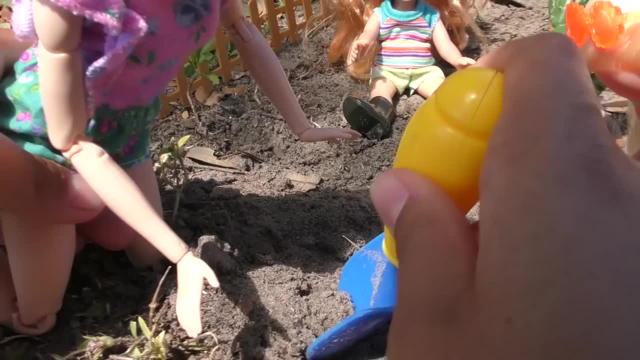 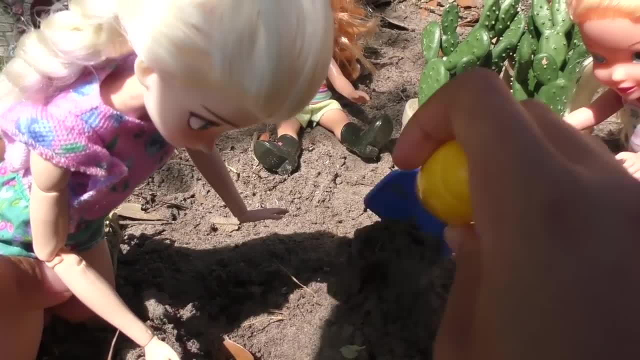 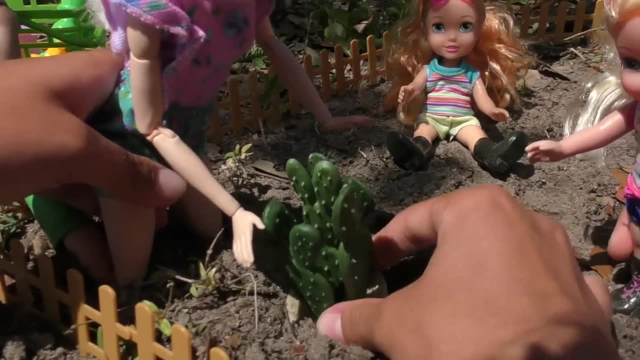 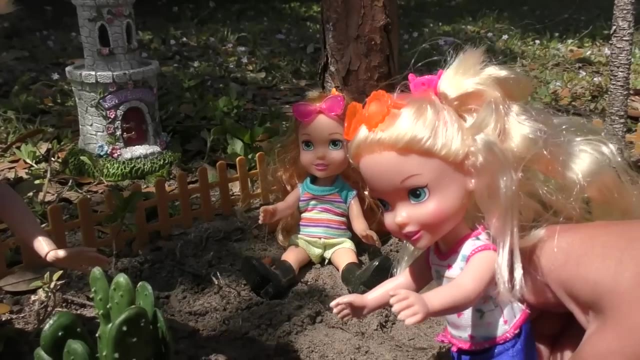 What's this? What's this? What's this enough for the plant to fit, dig deeper and then you put it in. are you gonna put it in with its pot? yep, this is a special kind of pot. when it when it rains, and when it rains, yes. well, when it rains, and over time it will melt and it's okay. 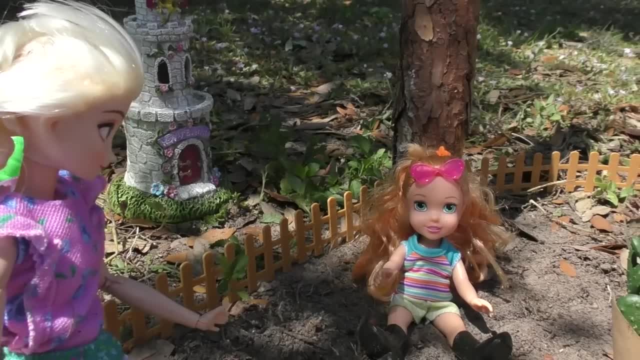 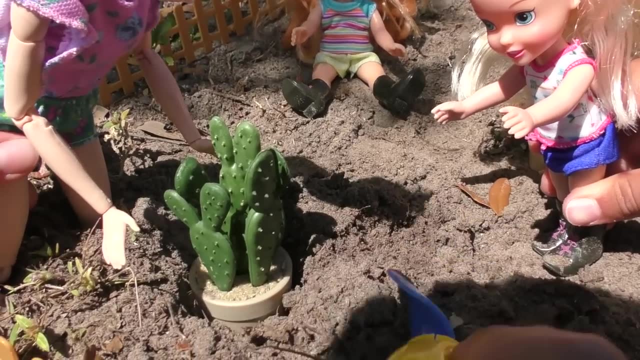 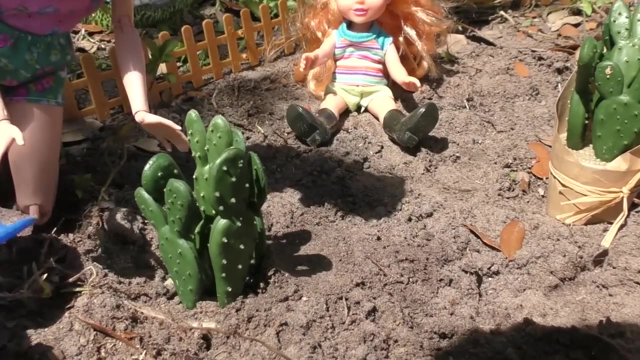 it's okay for the soil, so it's soil friendly. yep, it's biodegradable. really, it's a special kind of pot, nice, okay, and after you put it in, you put dirt around it like this. use your shovel. oh, it's moving. can I help from all sides? 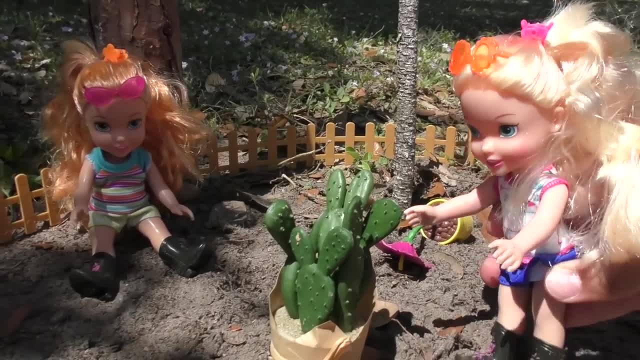 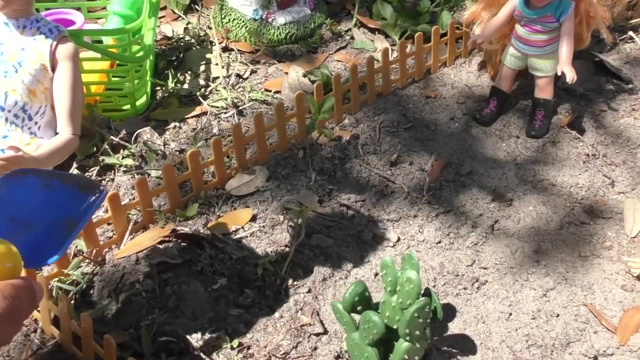 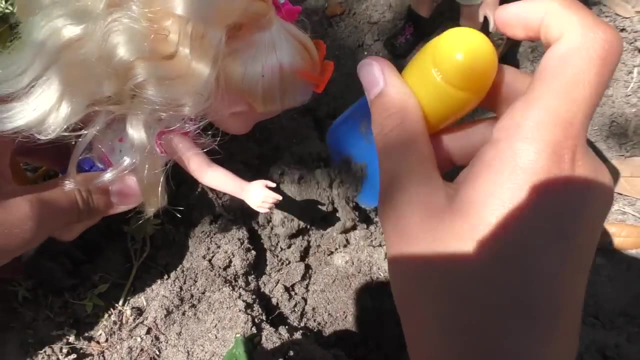 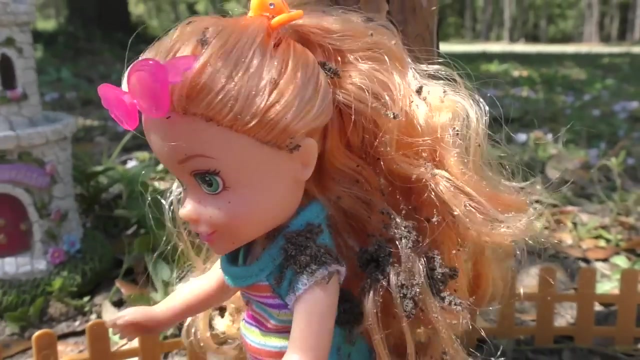 you can do the next one. okay, I can dig the hole and you can put it in, because I'm scared to touch the spikes. okay, sounds good to me. just put it over here. this will be the cactus area. okay, it's hard to dig, and dig and dig. Alciai, you got it in my hair and all my 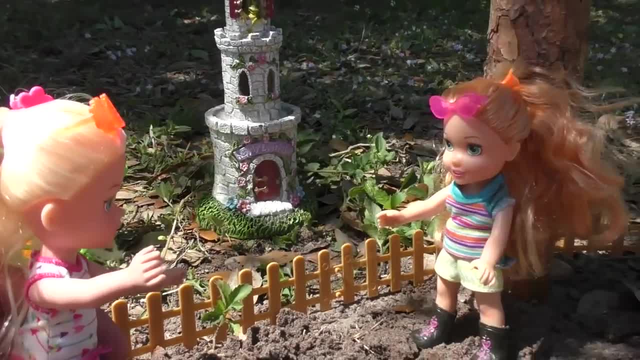 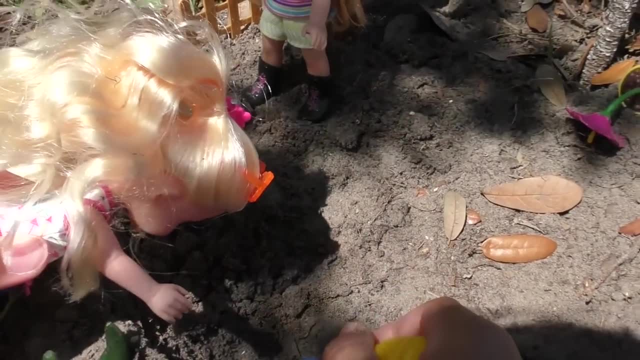 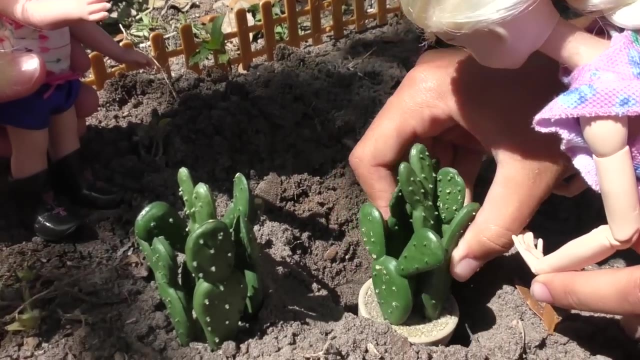 new clothes. shake it off. oops, sorry, I didn't mean to. don't worry, I'll be more careful. alright, scoop it more gently. I think that's good. let me see. is it too deep? nope, that's a good size. there we go, mm-hmm. 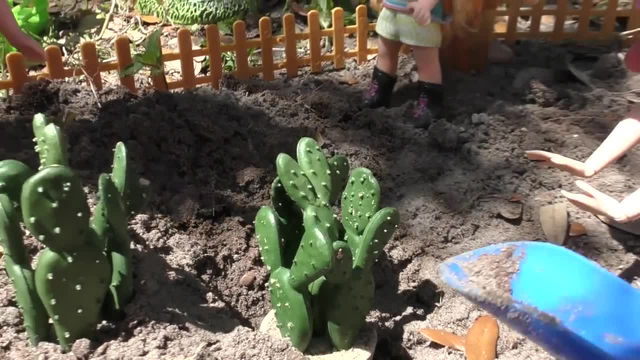 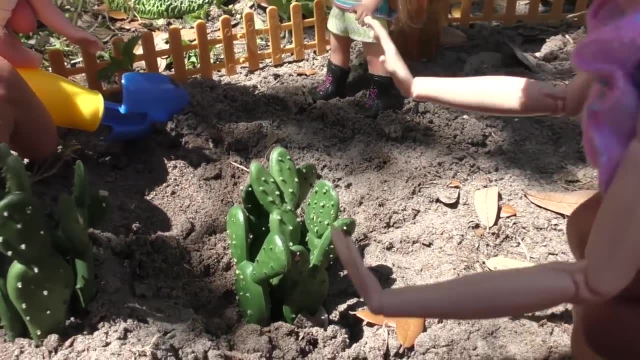 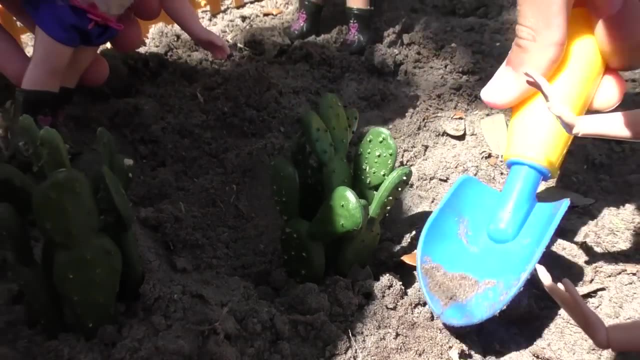 now you can put the soil in the pot. there we go oil on like this. Yep, just like that. Wait, is that too much? Yeah, maybe a bit too much? Okay, then I'll do it like this: Scoop it back down There, we go, Pat it out, And I. 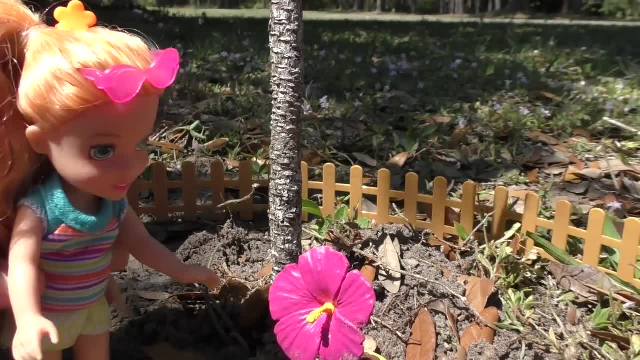 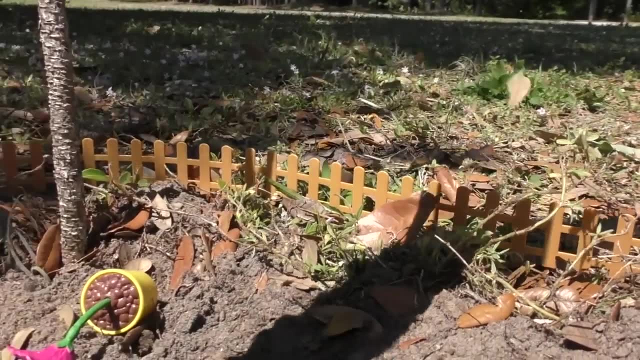 planted my first cactus. Oh, Biscuit, soon, you're going to be planted soon. Oh wait, where is Tangy? Oh, I know, Tangy, I'm coming. Oh, so windy, so windy. Oh, Elsia, did you. 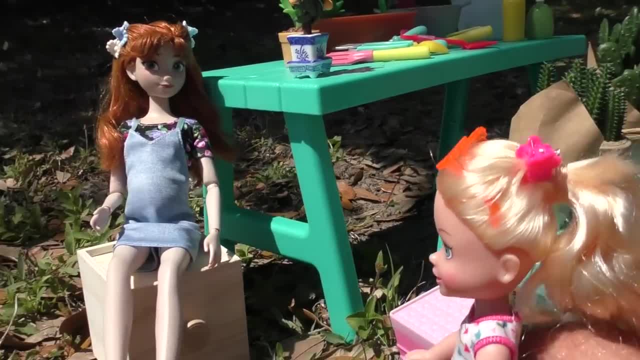 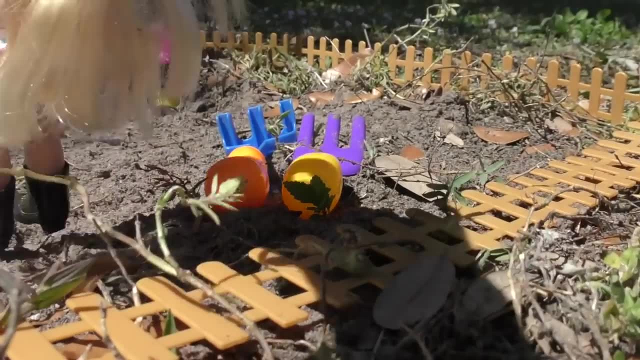 see what you did. The fence fell down. Tangy, here you are. Yes, Tangy, Tangy, my little orange tree, Elsia, you only care about Tangy. Look what you did. You knocked down two fences. 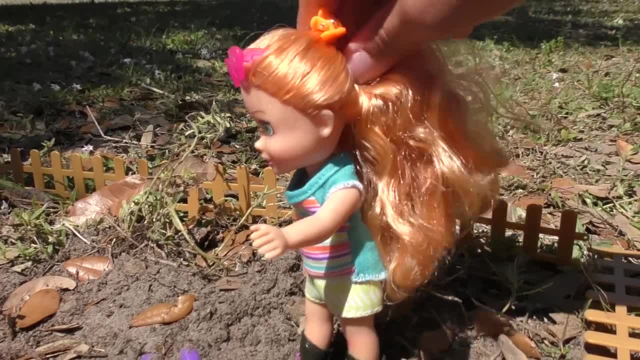 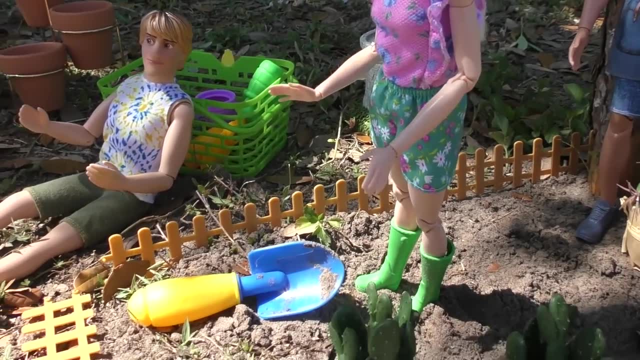 Oh, Tangy, yes, yes, yes, you are here. Yes, it's Here, but look what you did, Elsia. You knocked down this whole fence. Yes, Elsia, and when you went to get Tangy, this is what you did: You knocked down this fence over here, Didn't? 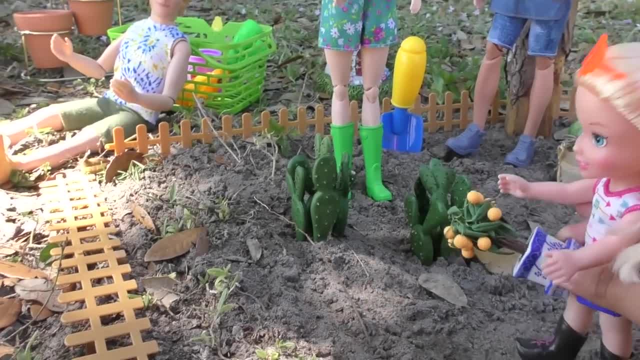 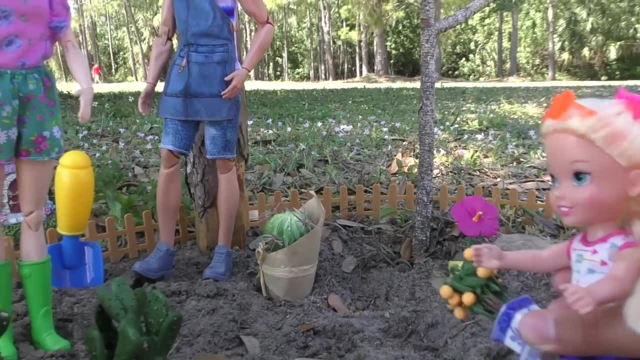 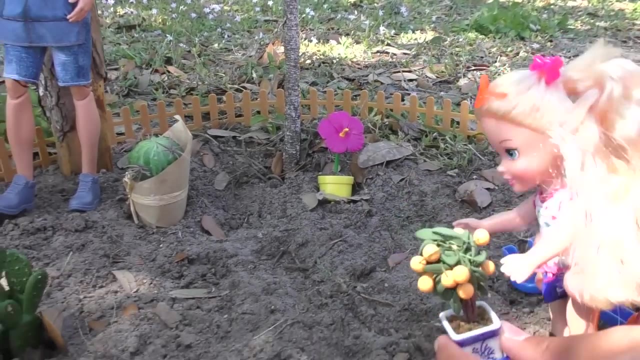 you hear me say: Oh sorry, I didn't even notice, And I think the wind even pushed me. Yeah right, No, I actually felt a strong wind. Well, it could be the wind too, but you still didn't watch out. Yes, that's true. Sorry about that. I'll pick it up, but please watch. 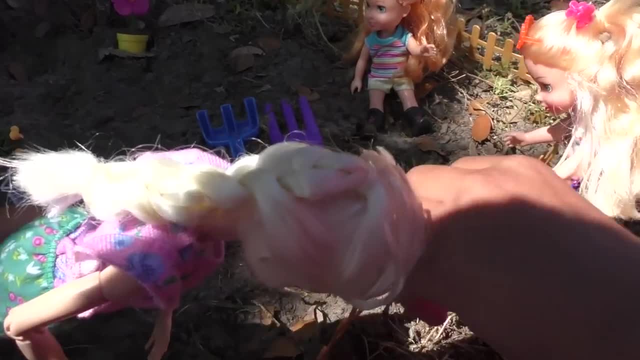 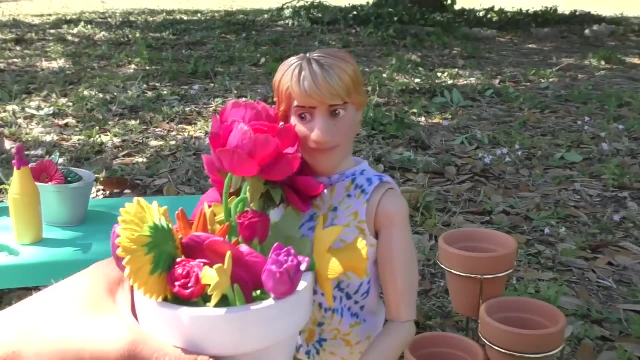 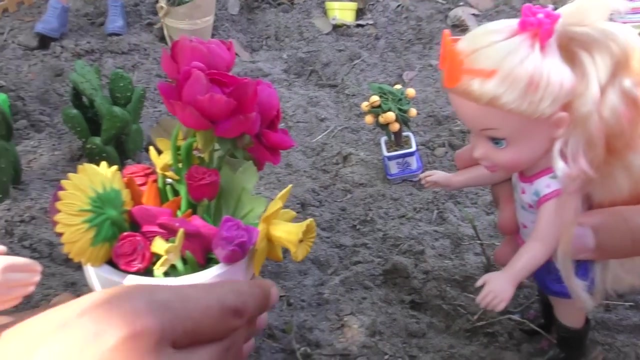 where you're going next time. Okay, I can help you. Here we go. Look what I have here. Who wants to plant them? Look at all the flowers, girls. Whoa so amazing. So you girls can plant them everywhere in the patch, all right, One by one. Yes. 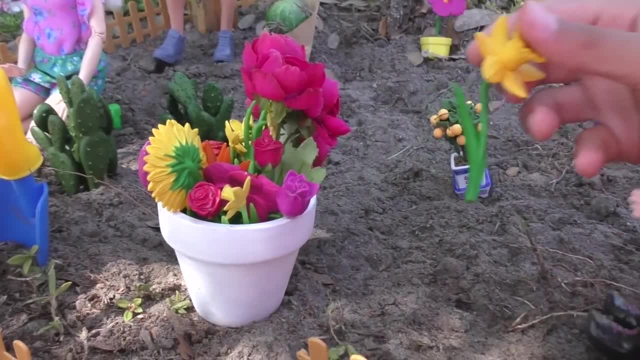 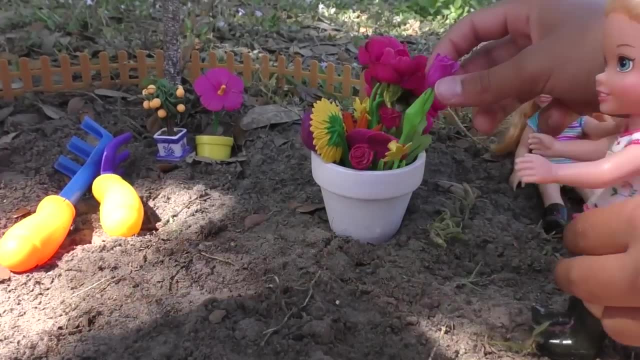 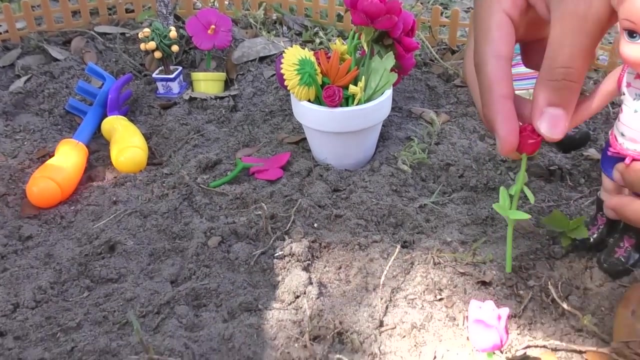 and we don't even need to dig because they have small stems. Let's make flower lane A beautiful yellow one, And we can add a purple rose And whoop, They're going to grow so tall. Oops, Oh, this one. 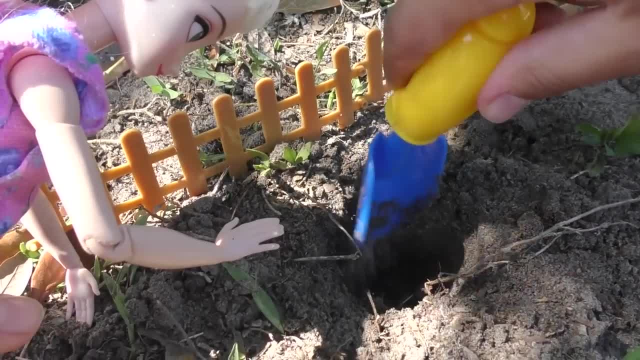 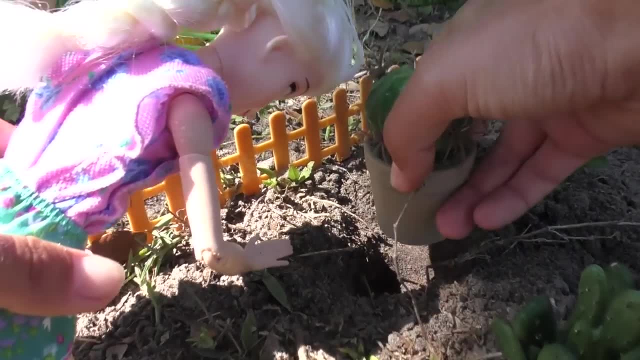 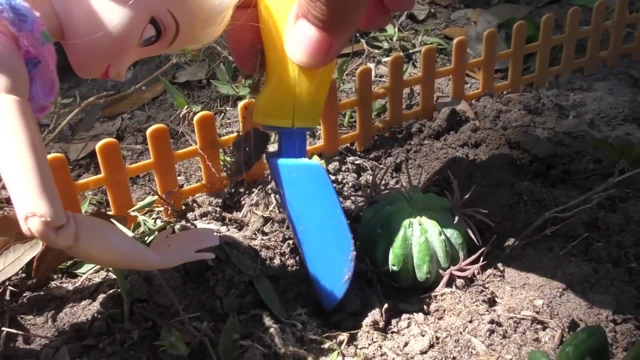 fell. Come on, Anya, let's go. Look how deep I dug this hole. girls, Whoa. Okay, we're going to put a round cactus in there, Pat to the dirt, And the next one, you girls work. 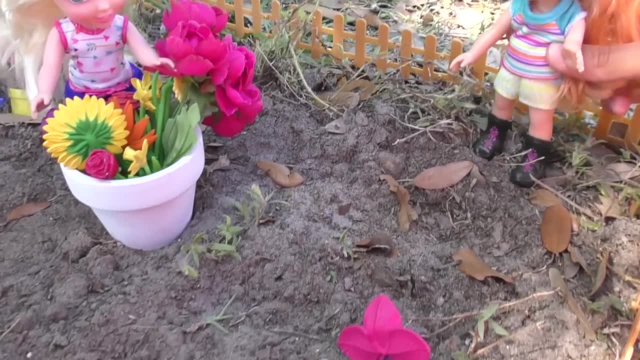 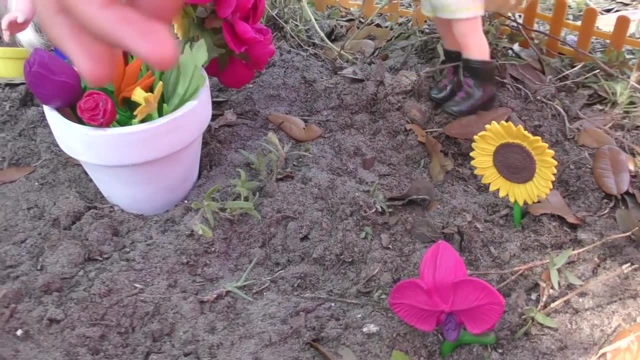 on the floor. I think I'll get the flowers and I'll work here. We are almost done with first row Sunflower, Mommy's favorite. Here we go, And then one more, This little yellow one, Look, look, look, We're finished. Look, Yellow. 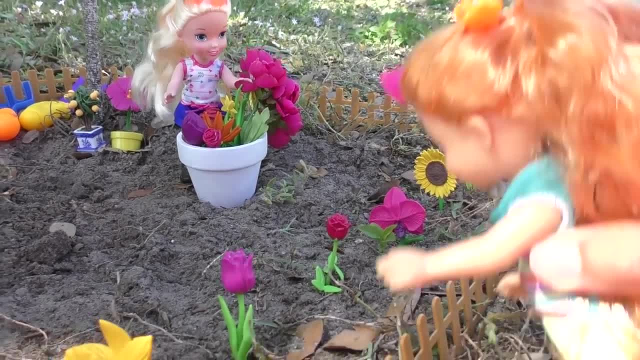 purple, pink, pink, yellow, yellow, We're done, We're done. And look, One, two, three, four, five, six, Six, Look Mommy, Look Mommy, I can see them. girls, I like it. 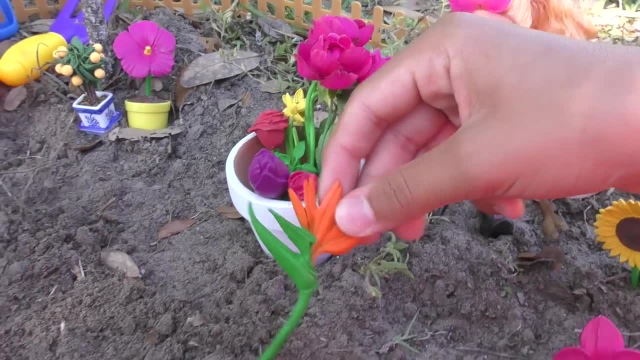 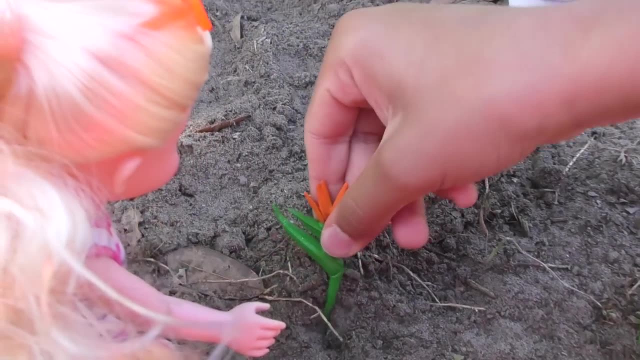 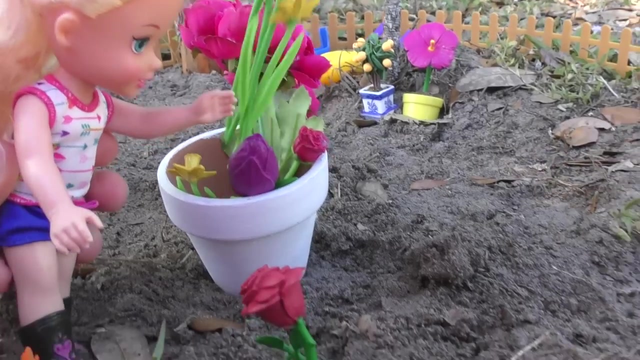 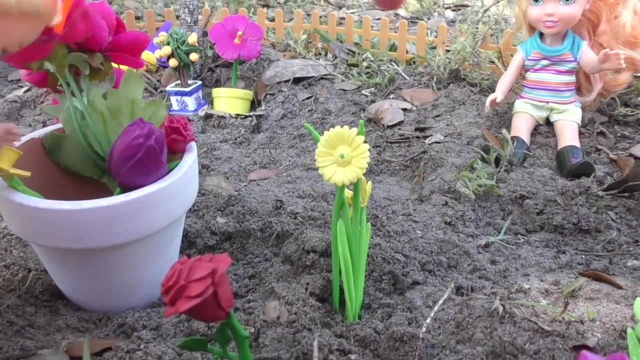 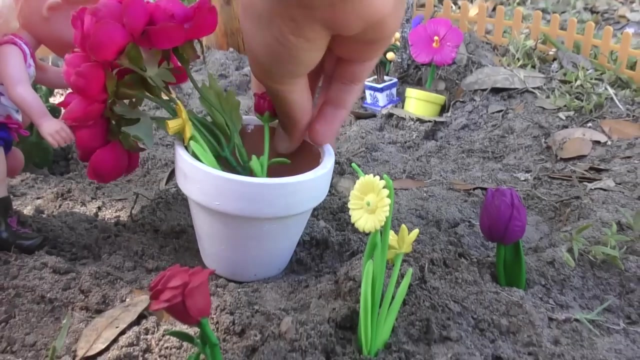 Yes, Going good. Orange one, the pond flower- oh, this is gonna look so bright and colorful- oh no, it keeps falling. i need some extra soil. big pink rose daisy- oh, this is a really big one. and purple tulip- oh no, the pot of flowers. are they okay? oh yes, they are. where are we? 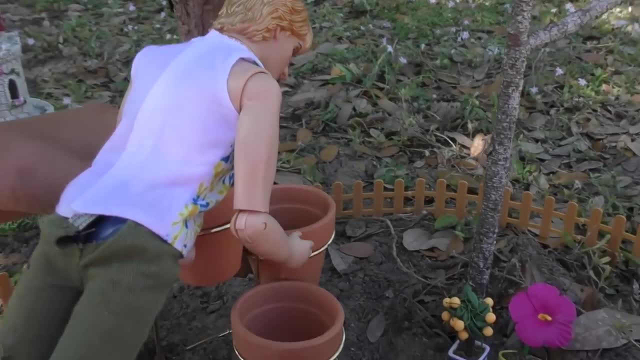 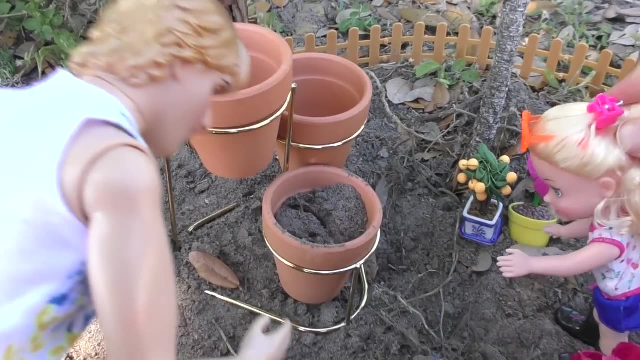 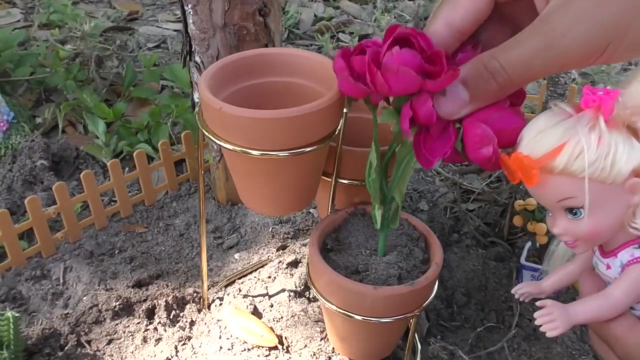 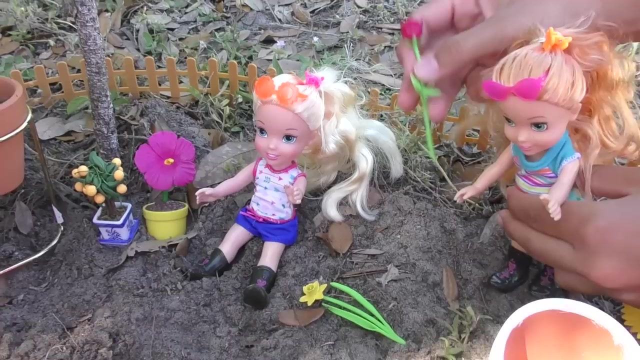 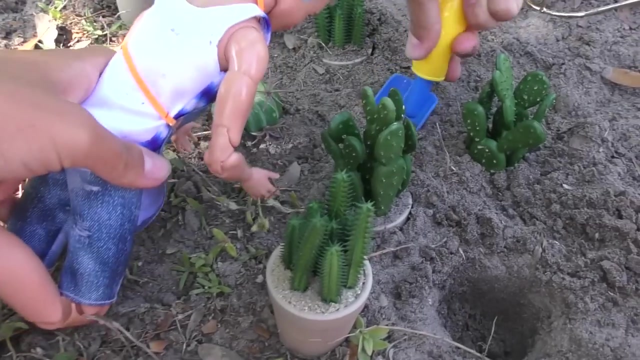 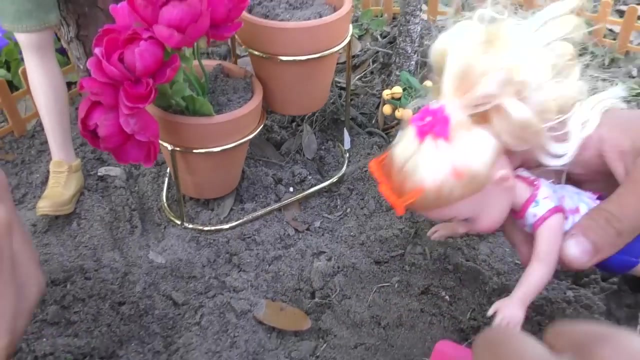 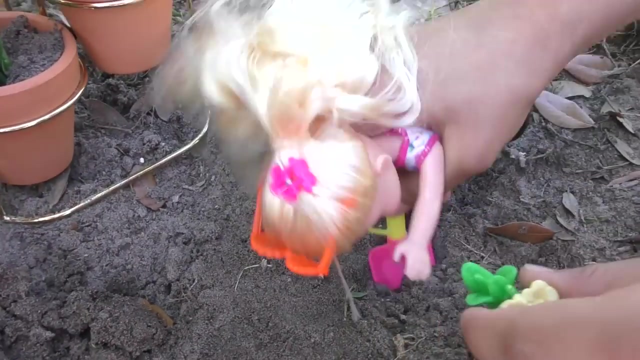 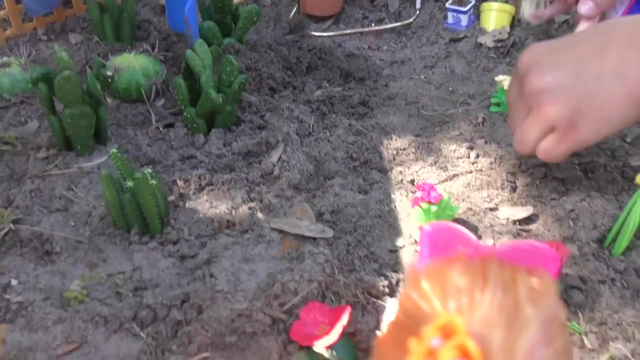 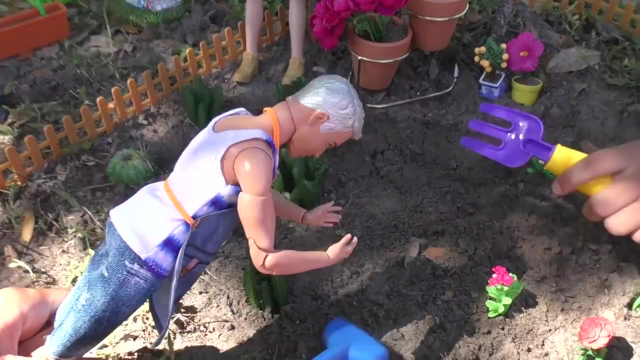 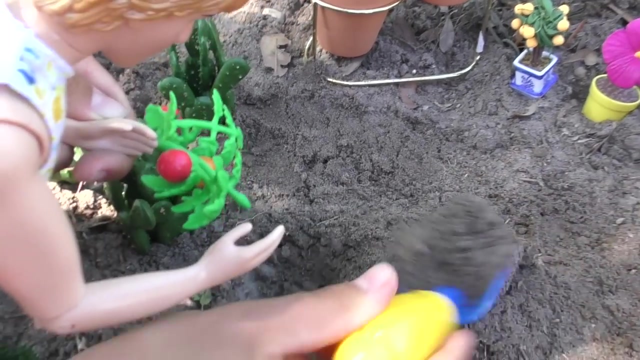 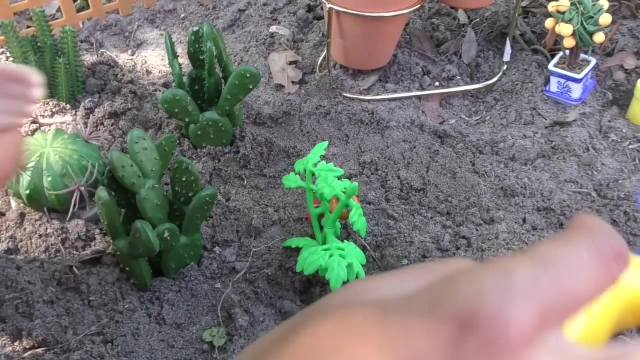 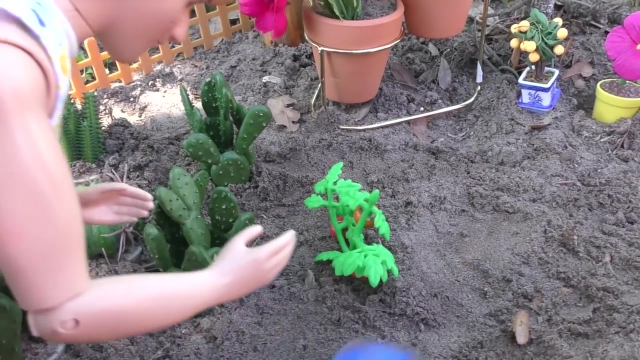 gonna put this one. use this, girls. oh yeah, the big pots can't wait. it's gonna be like a floating display. can i put it in now? yep, good job, beautiful. so so, so, on time for my tomato. perfect, we will have fresh tomatoes. the garden is ready. it's all finished. look at all the plants. we did a great job. our pet plants- they. 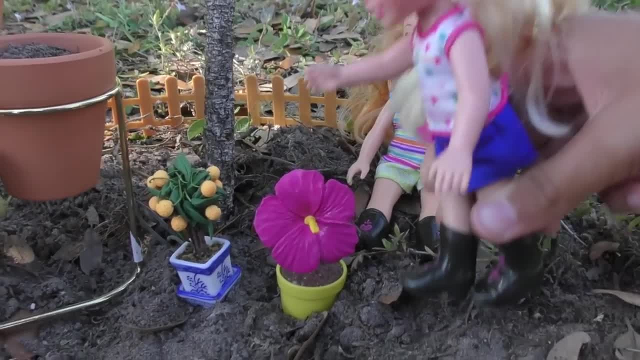 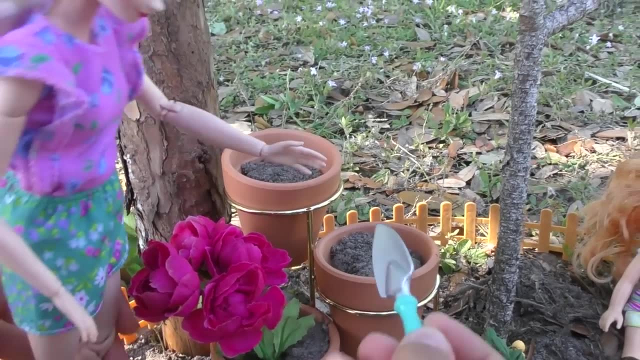 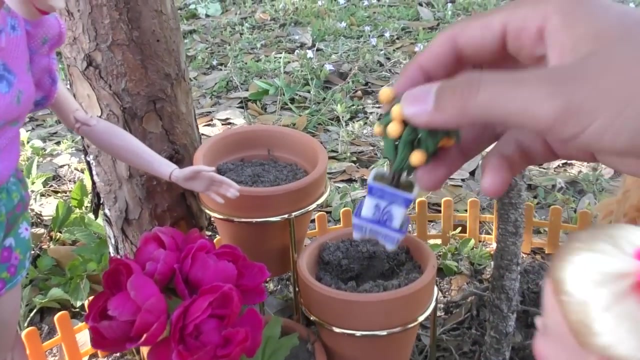 our pet plants, they know how to grow them. our pet plants, they know how to grow them. we need to go in the pots. we forgot them. well, that will be easy and we're going to use the tiny shovel to just make a little hole right there. just dig a little tangy. welcome to your new pot home. 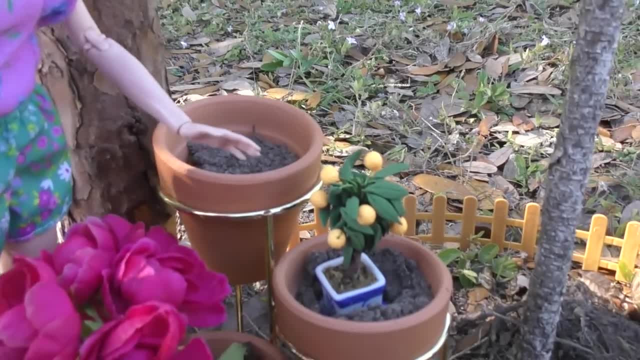 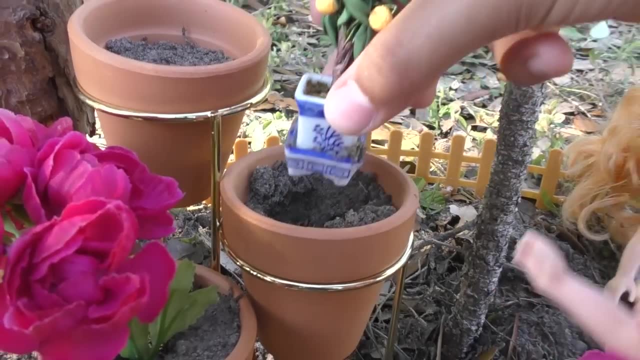 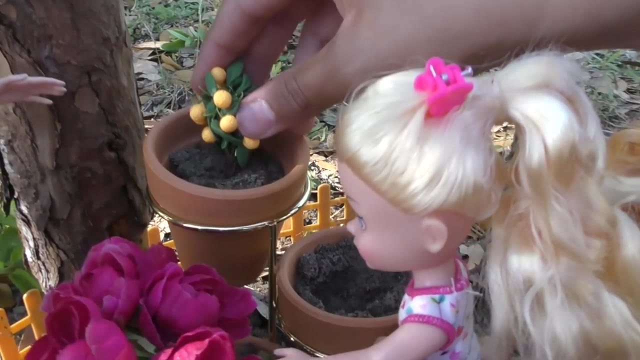 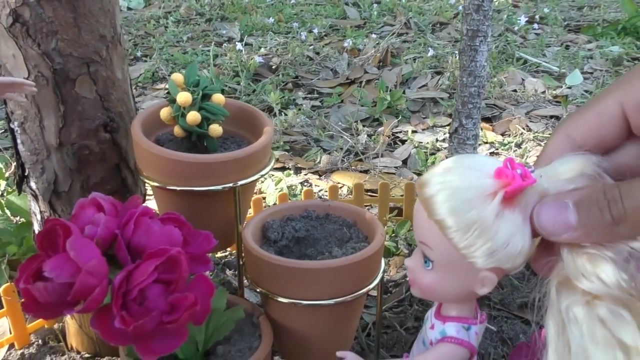 yes, there you go. oh no, no, no, elsia, that pot it's not degradable. oh, oh yeah, all right, then we have to take it out. yep, there we go, tangy out from your old pot, oop, out from your old pot into the top view. oh, you're putting in the top? yes, because i want it to see the nice view up high. the best um a and the best um a. pardon me, elsia, i think a biscuit need to have the best view, not tangy. the tree there for tangy can go and biscuit, come on up for the best view ever, cause you deserve it, not tangy. 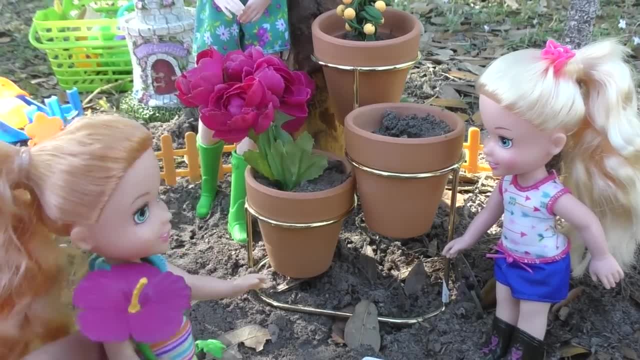 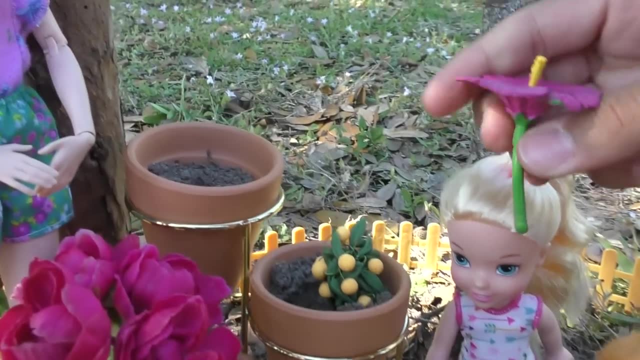 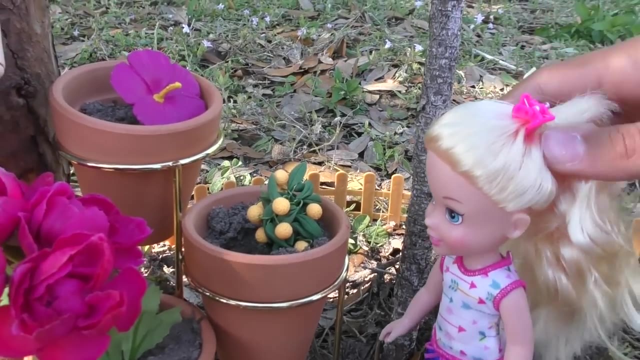 i think a biscuit needs to have the best view, not tangy the tree. therefore, tangy can go there and biscuit, come on up for the best view ever, because you deserve it. not tangy anya? hey, that was pretty fun. supposed to be tangy spot and you put soil on its oranges. look at that, mommy. 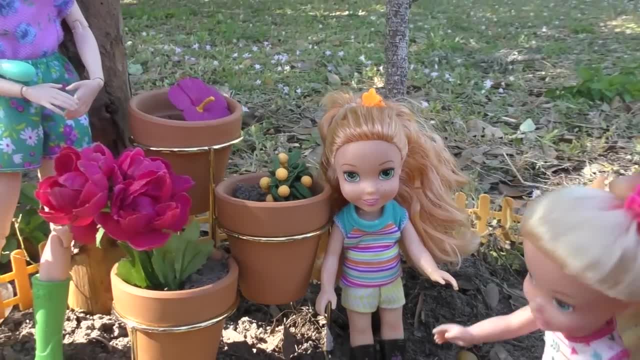 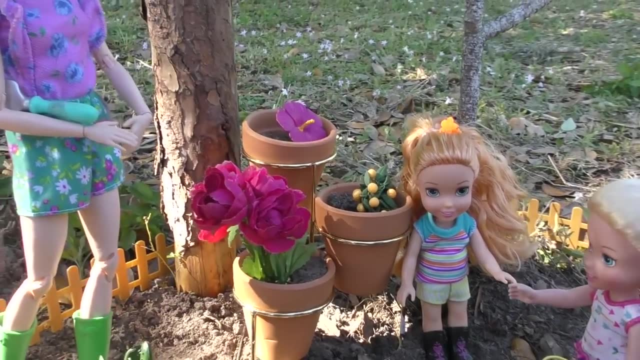 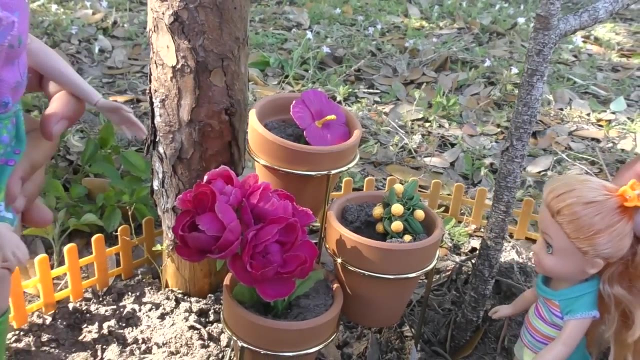 did you see what she did, poor tangy? she needs to get the best view and, by the way, I was the one to choose first. girls, girls, we don't. we don't need to argue over this. I think it's fine like this. what's wrong with this? well, I was the 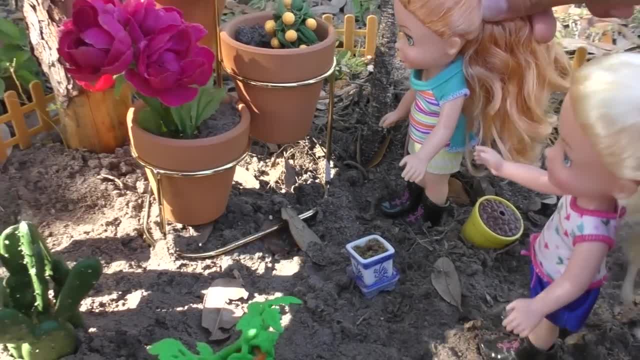 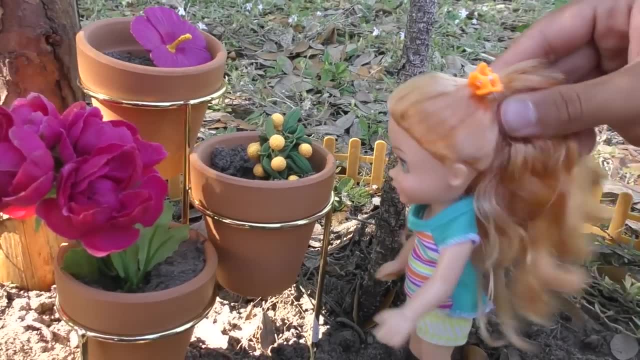 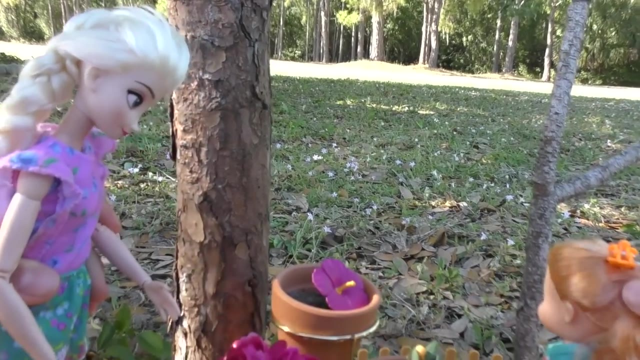 one who got to pick first. so that isn't fair. hmm well, I guess hell see how you do have a point. yes, you don't even understand Elsa, it's just the view doesn't really matter, they're both the same. I guess they could have a pretty. 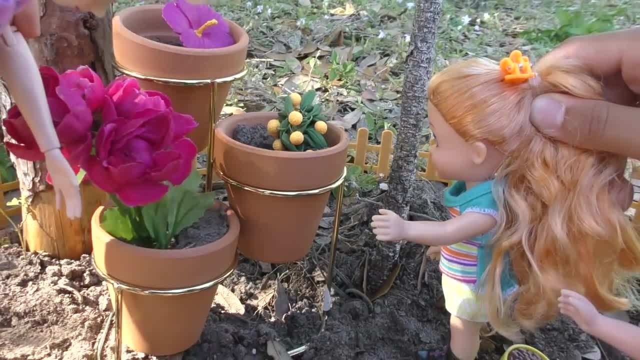 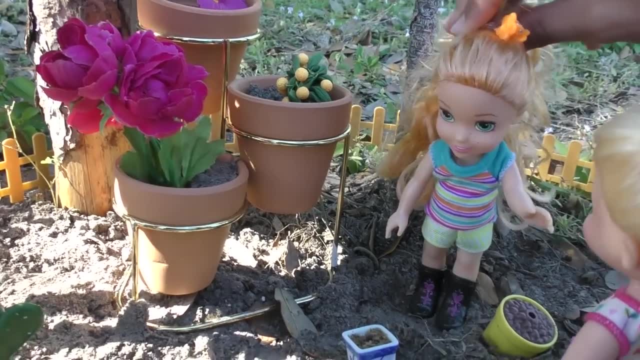 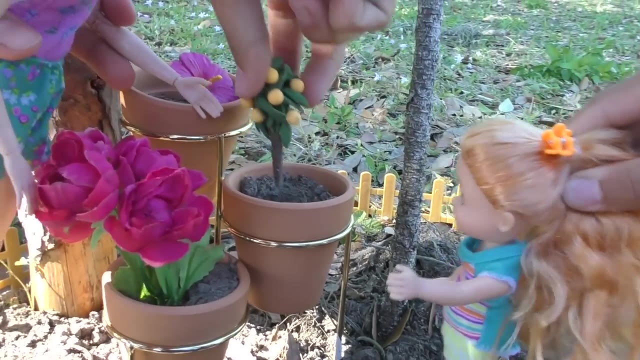 good, equal view. yeah, they're both high, see, this one is the lowest one, okay, well, so how do you say to Elsia: okay, I'll see, ya, I'm sorry you. you can have your spot back and they, they can actually see a nice windy view. 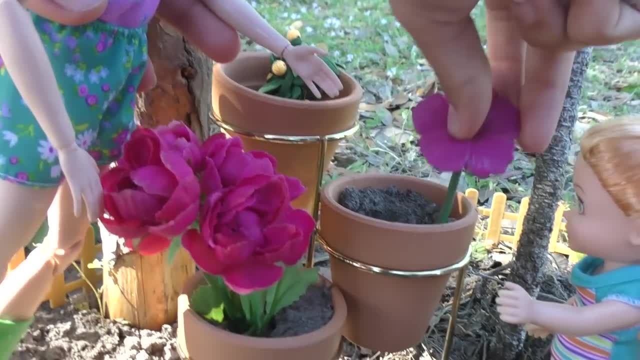 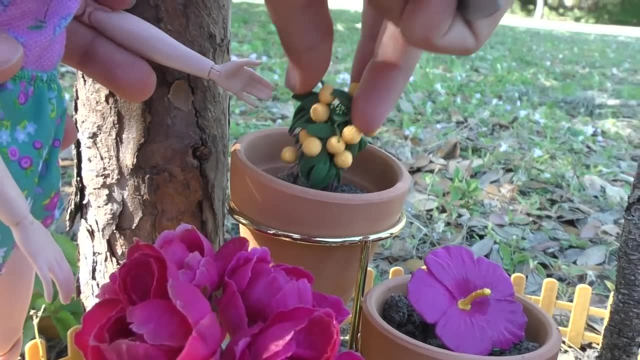 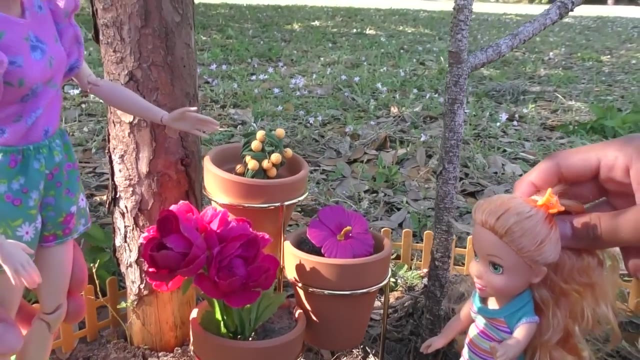 anyway, both here, I'll switch them around and you dust off the dirt off of its oranges too. yep, so are you both happy now? actually? yeah, we like it this way. you know what? huh, the last thing to do is water all the flowers. oh yeah, to give. 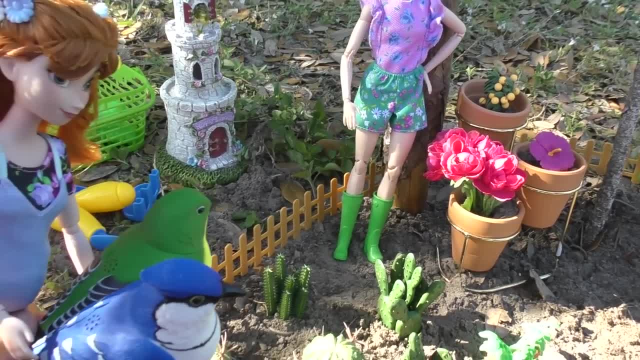 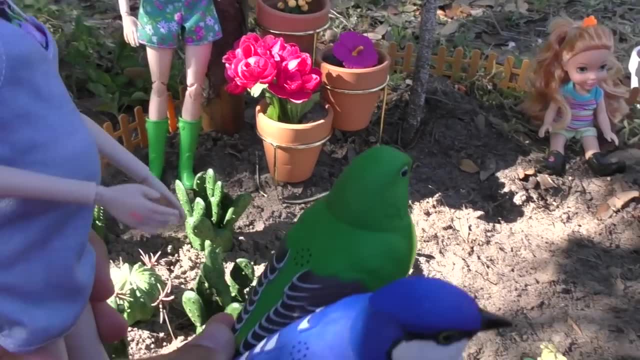 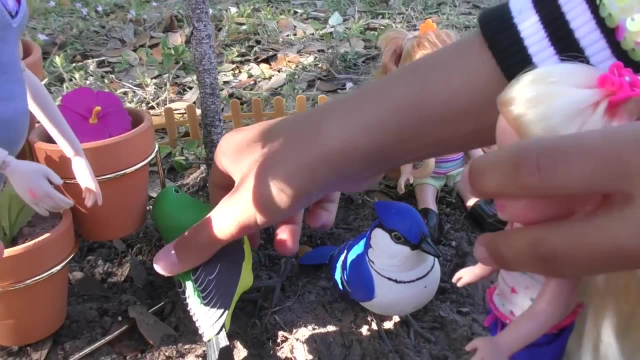 them the food they need. let's go, let's go. don't forget about the cutest part to add to the garden: the birds. remember the cute little birds and they chirp right. yeah, we can put them over here to guard your flowers. yay, this one can stay here. 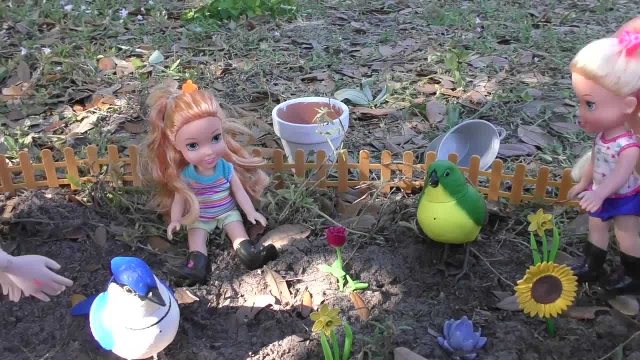 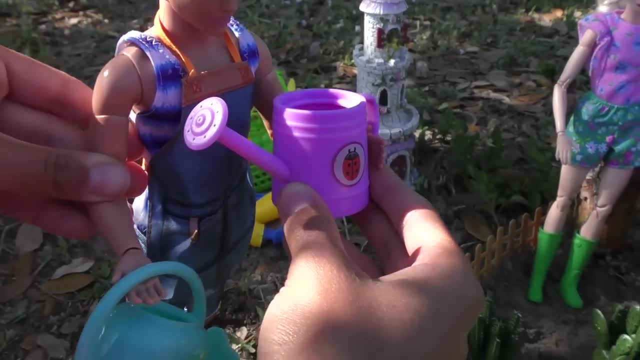 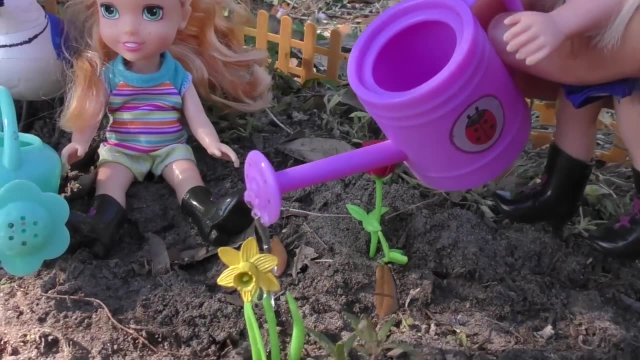 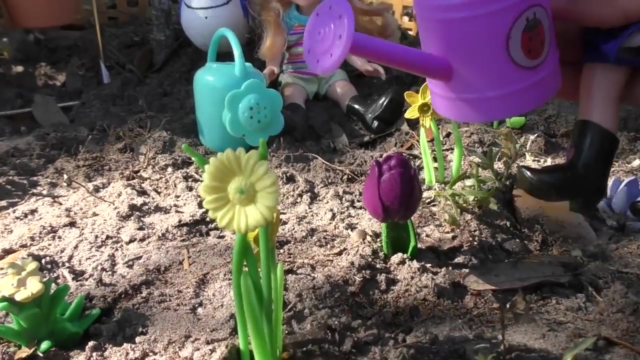 yes, and we should name them. this one can be lime, and what about the other, Anya frosty? here comes the water, they're all filled up watering cans. who wants the? Who wants the ladybug one? Me, Here we go. Next one, Elsia, you missed the purple one, Oh yeah. 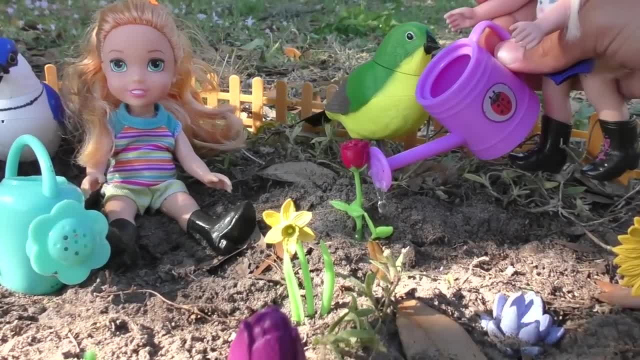 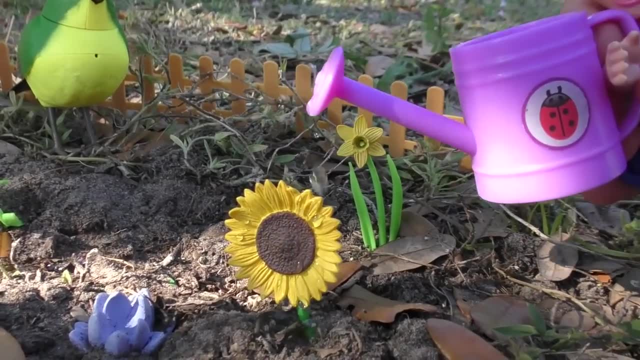 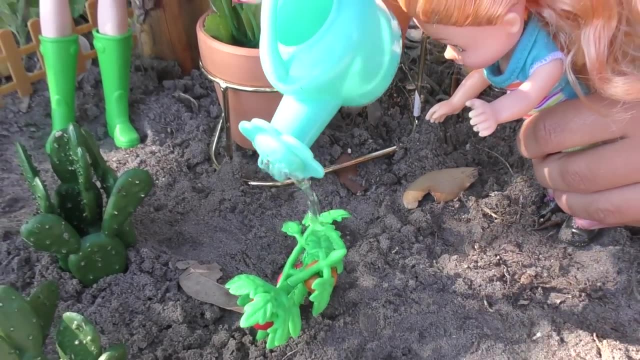 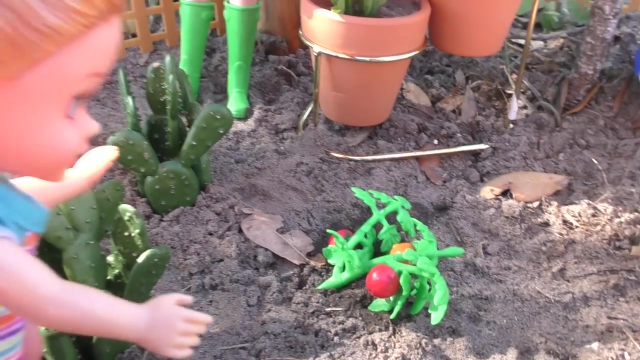 Alright, and now this little rose here. This is fun. I like this Sunflower, Little yellow flower. The tomatoes: Here we go. The tomatoes fell over because you put too much water, Anya, look what you did. Sorry, sorry, Here I'll arrange it. 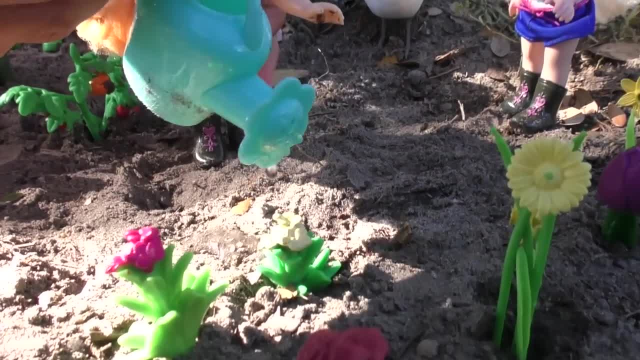 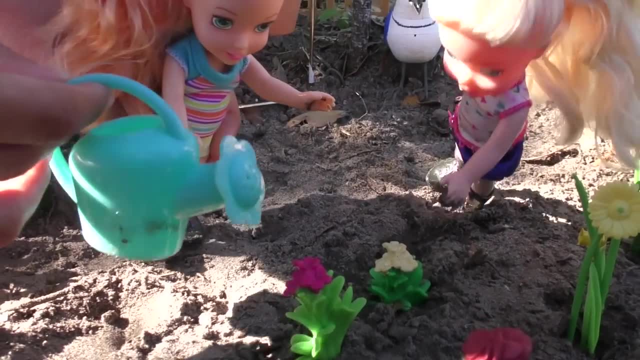 for you. I'll make sure to be careful. Okay, this one, Anya, where are you putting the water? See, look It's way over here. Needs to be on the flower. Sorry, sorry, I'll get it right, Don't worry. 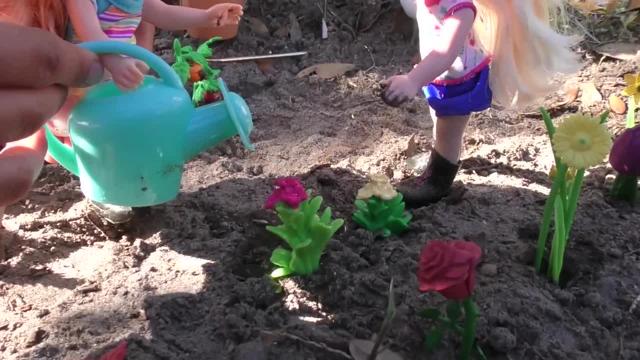 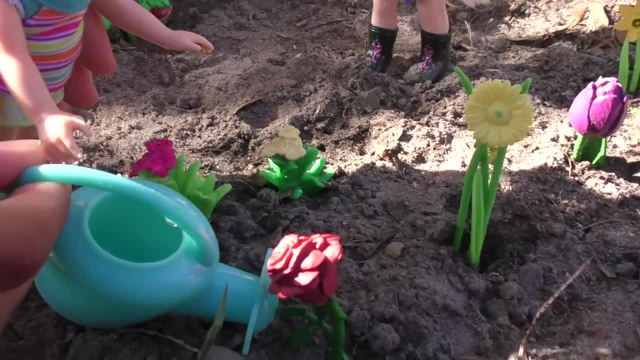 Not right on top. On top of it, Anya, Elsia, Elsia. it's okay, She's just doing it a different way. Fine, To the root. if that's how you want it, Okay, right there, Right there. No, Anya, don't put it. 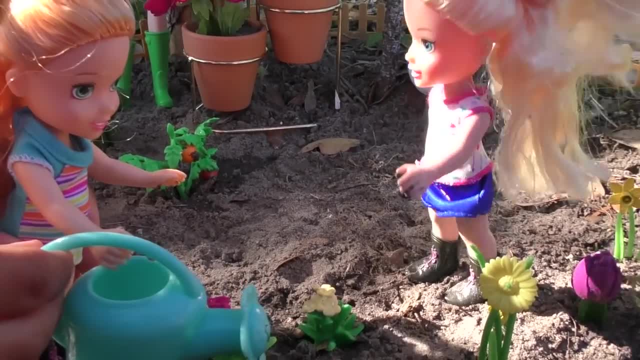 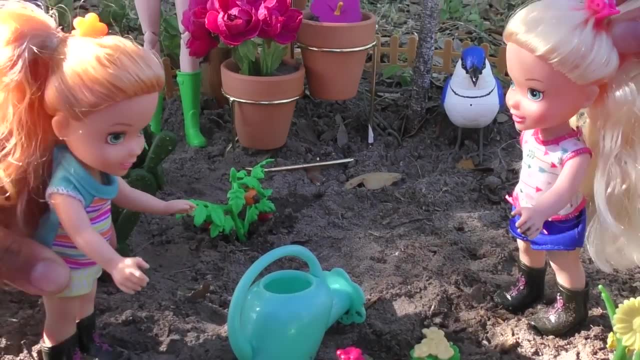 Don't put it. Put the picture right on the dirt. You don't do that. Well, you said the roots. Show me how to do it then. if you're so smart, This is just the correct way how to do it. Watch and learn. 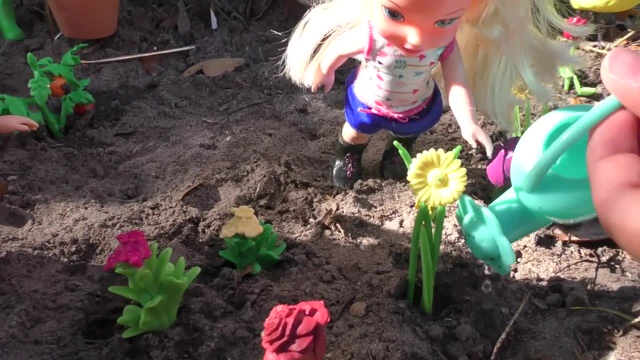 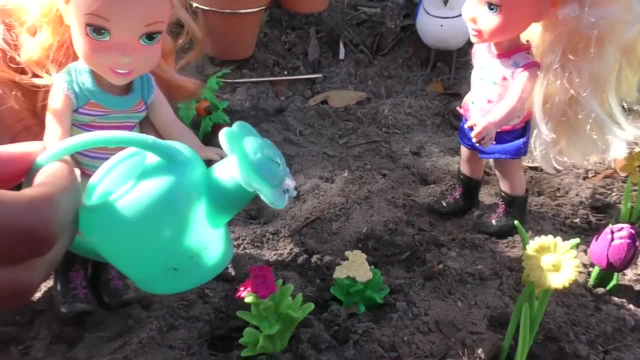 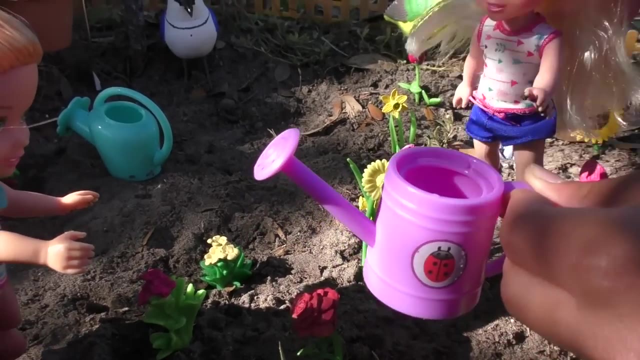 Ready A bit above the roots, Then just go Just like that. Hmm, All right, then I'll try it. then See if I do it good this time. Oh no, Is there any more? Oops, I need a refill. Oh wait, You can use mine. 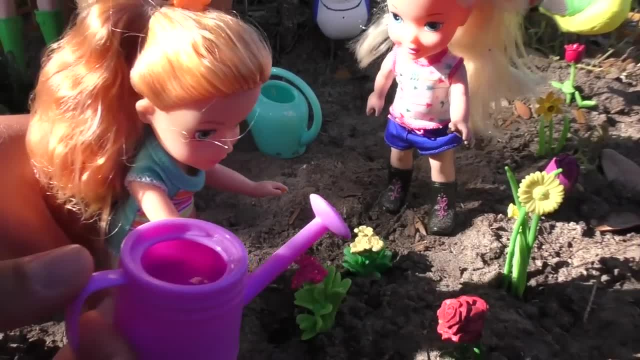 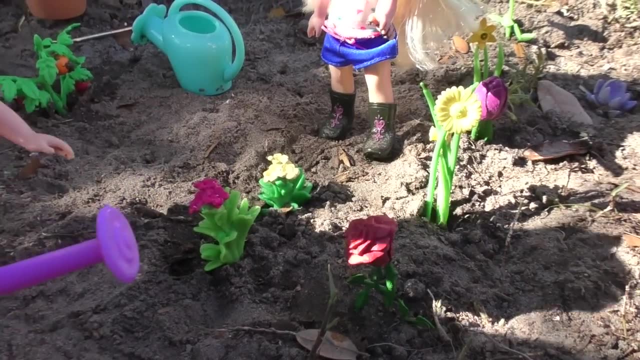 I have a lot more. All right, Let me try this one. Oh yep, Oh yeah, You did it good, Great job. Oh yeah, It is fun to do. I can't wait to do it that way. 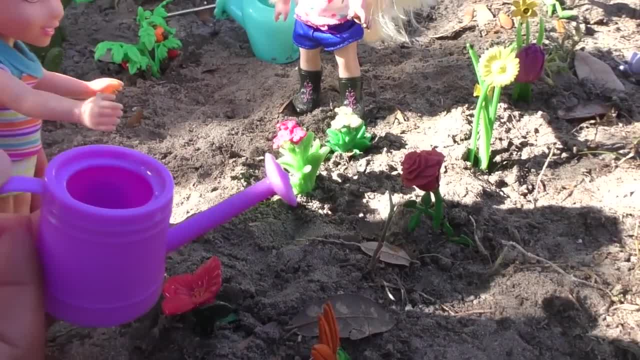 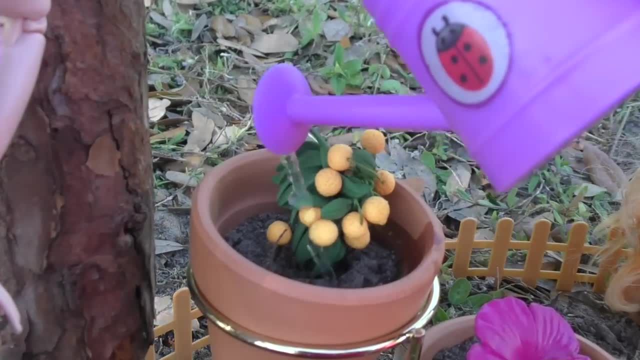 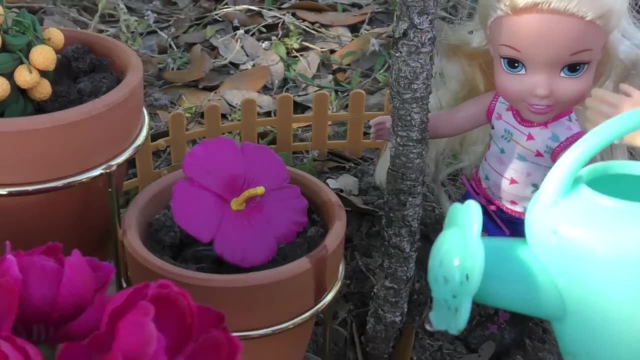 Mm-hmm, Woo-hoo, Oh, There we go. All right, Tangie Water is coming for you. Water for Tangie Biscuit. here's a fresh drink for you. There you go. I love hearing the birds chirp. 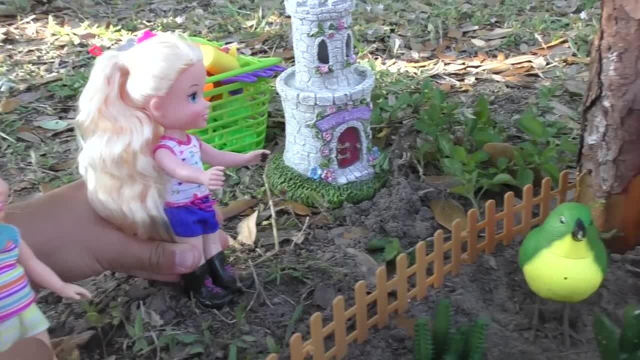 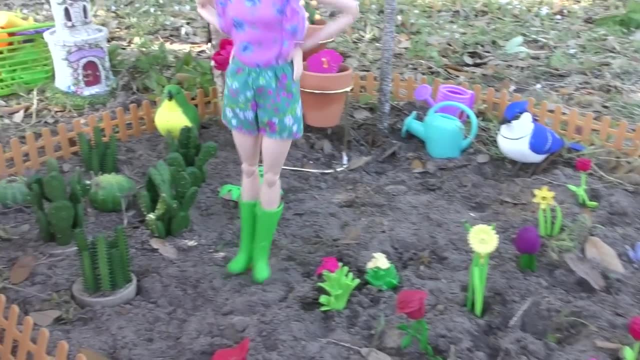 Oh, I'm kind of thirsty, to be honest. Yeah, let's take a break, girls, We're done for today. Look at all this work we did. Yup, So beautiful. All right, Let's go. I'm so thirsty. 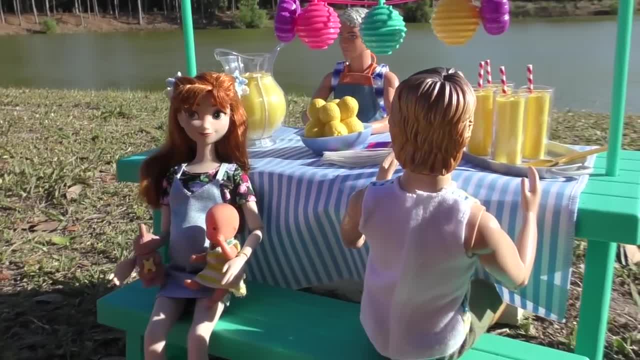 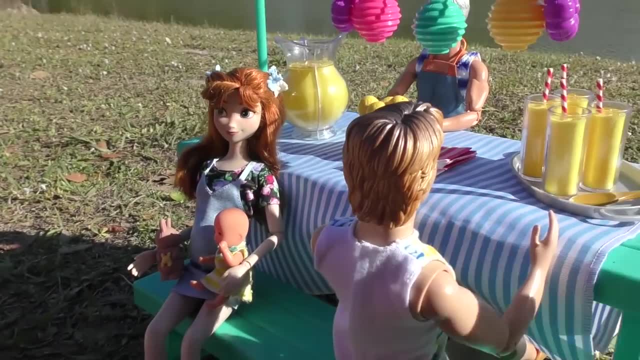 Guess what? Huh, Anna, you got lemonade. Yup, Lemonade. Yes, What a nice surprise. Thank you, Mommy. Yes, Yes, Thank you, Anna, I'll go on this side. Lemonade, Lemonade After a hard day's work. 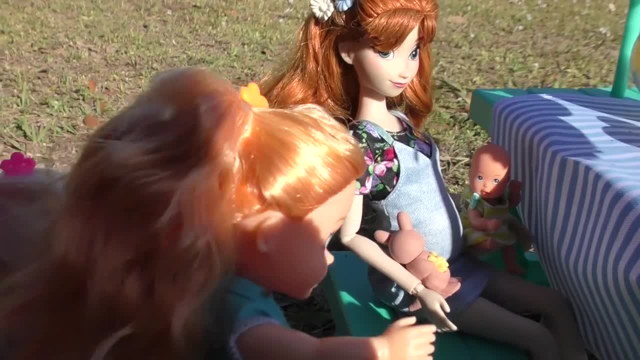 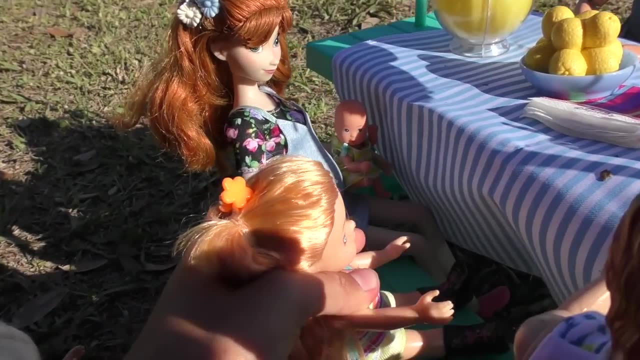 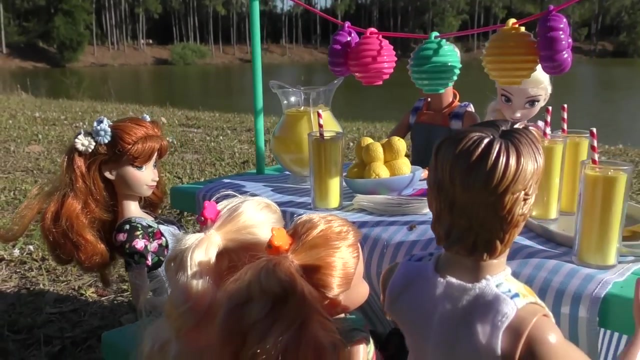 Aw, Hey, Snowflake, Did you see us planting? Aw, And you have your kangaroo toy I got you. Mm-hmm. I'm gonna sit with Anya Lemonade, Mm yummy, What a nice spring day. 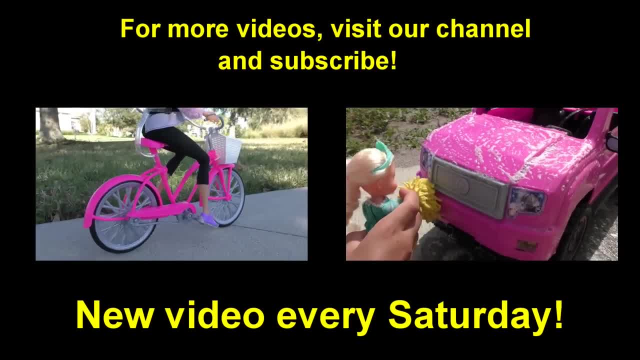 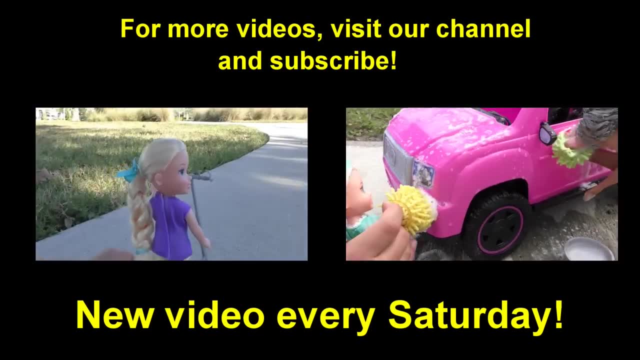 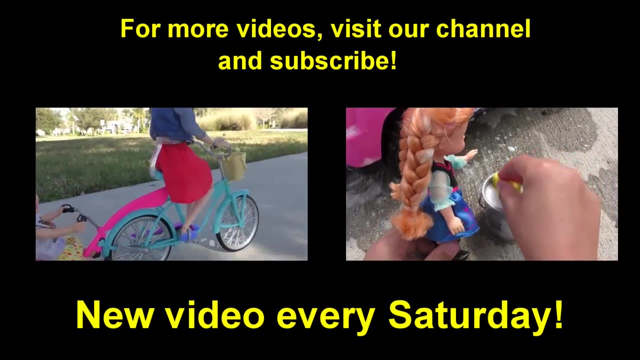 Love it For more videos. go to our channel and subscribe And join the Rubber soreless quad nation Right? Hey, Colton, what are you looking at? 제일 굉장히對, You have to run fast to make contact properly. I'm coming, I'm coming, You know I will. Okay, all right, Thanks. Yeah, See you tomorrow. Bye, Bye-bye, Take care. Bye. We're getting ready for the dive. Yep, I gotta put it in my backpack so I can go for the fun. 발� didn't we go all the way. boo, I just realized you forgot something. I haven't put him fine or anything. he's got this.